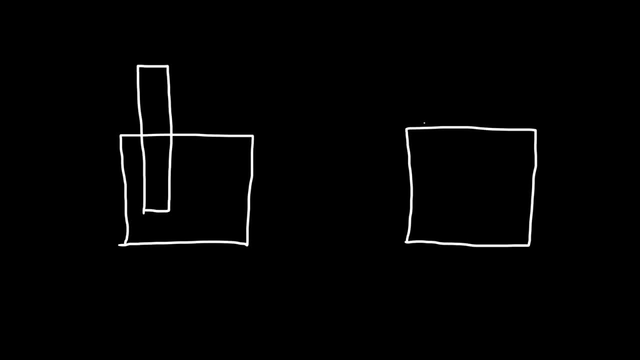 electrode. an electrode is simply a metal. metals conduct electricity. now the metals have to be in contact with a solution. so this is going to be a zinc metal and this is going to be copper metal. so that's the copper electrode. the half-cell on the left is going to contain a solution of zinc sulfate and 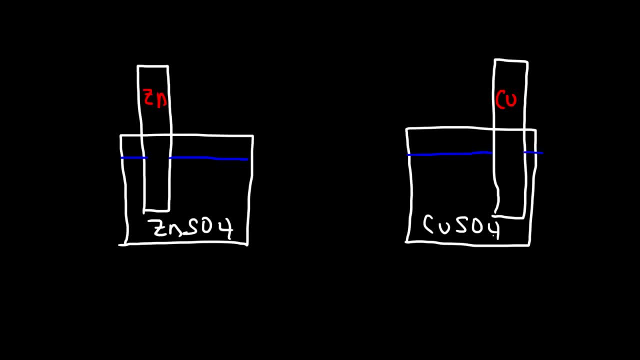 for the one on the right is going to contain the solution of copper sulfate. now I'm going to connect each electrode to a wire and to a light bulb, or you could use a meter if you want. now we also need a salt bridge to prevent the buildup of charge between these two solutions. 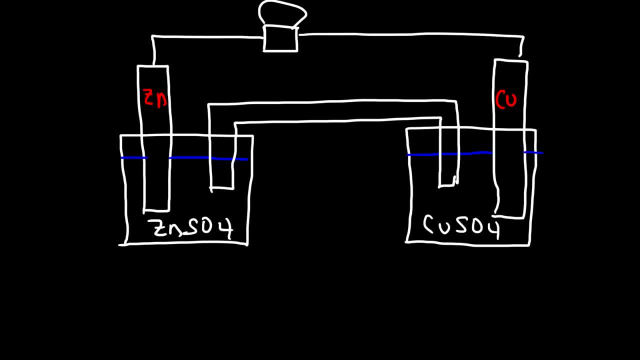 Now let's talk about what's gonna happen. Copper has a very strong tendency to accept or acquire electrons. Zinc wants to give it away. So zinc is going to lose two electrons per atom, and so it's going to turn into the plus 2 or the 2 plus ion. 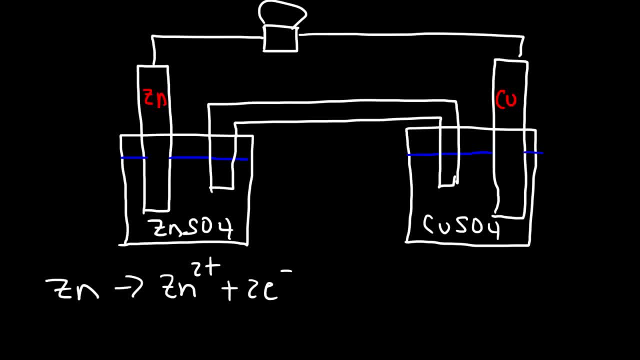 Now, whenever a metal loses electrons, it's undergoing oxidation, and you need to know that oxidation always occurs at the anode. So zinc is the anode. The other electrode has to be the cathode. Reduction occurs at the cathode. So remember, oxidation is the loss of electrons and reduction is the gain of. 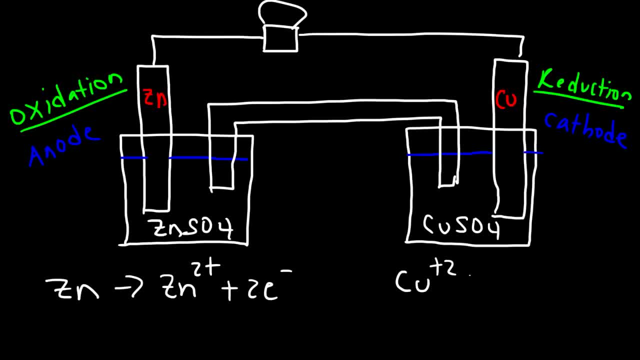 electrons. So at the cathode copper ions will acquire electrons to turn into copper metal. So if you look at the oxidation states, the oxidation state of any pure element in its natural state is 0.. So for zinc the oxidation state increases from 0 to plus 2 or 2 plus. 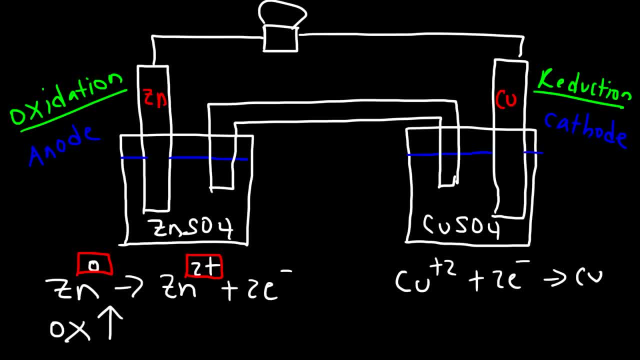 So anytime the oxidation number increases, the substance is undergoing oxidation. It's losing electrons. In the case of copper, notice that it goes from plus 2 to 0. So the copper 2 plus ion is being reduced because the oxidation number is decreasing. It's acquiring electrons. So these two reactions are: 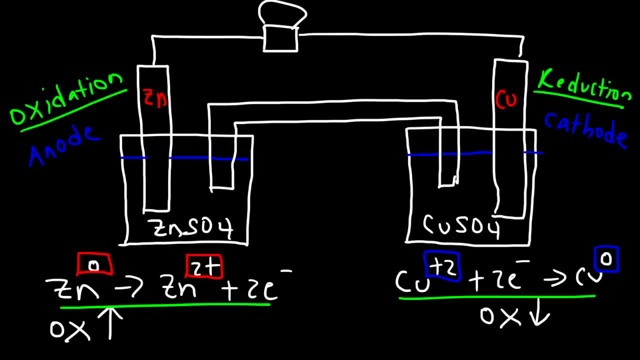 known as half reactions, and you can easily tell if a half reaction is an oxidation reaction or if it's a reduction reaction. And here's how you tell: Look at the electrons, specifically where they are relative to the arrow. If the electrons are on the right side, you have 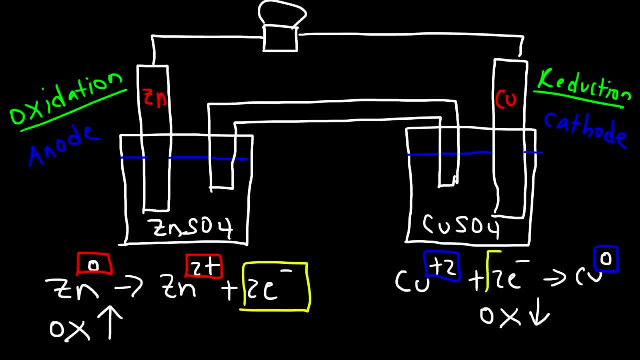 an oxidation reaction. If the electrons are on the left side, you have a reduction reaction, And so that's a quick and simple way to determine if a half reaction is a reduction reaction or an oxidation reaction. But keep this in mind: oxidation always occurs at the anode and reduction occurs at the cathode. Now we 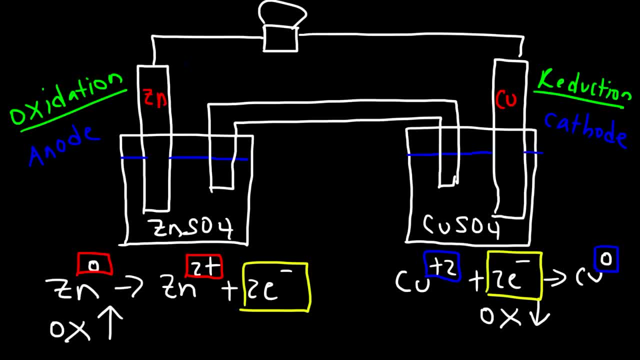 know that zinc is giving away electrons, So electrons will always flow from the anode towards the cathode. So because the electrons are leaving the anode, the anode is negatively charged. Electrons always leave the negative terminal of a battery and flow towards the positive terminal of a battery. So the cathode is 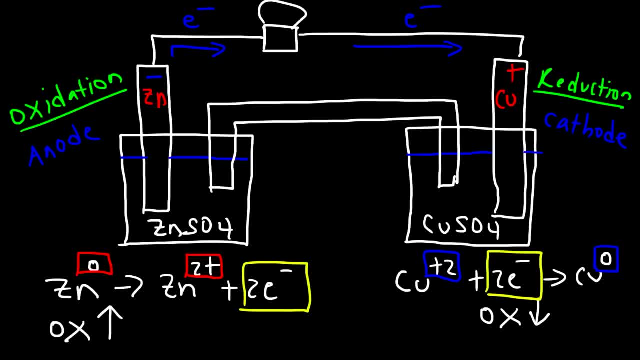 positively charged because the electrons are flowing to it. Now, as electrons flow through the light bulb, the light bulb is going to light up, provided if this battery has enough energy to light up the light bulb. Now, what's happening at the interface between the electrode and the solution? specifically, 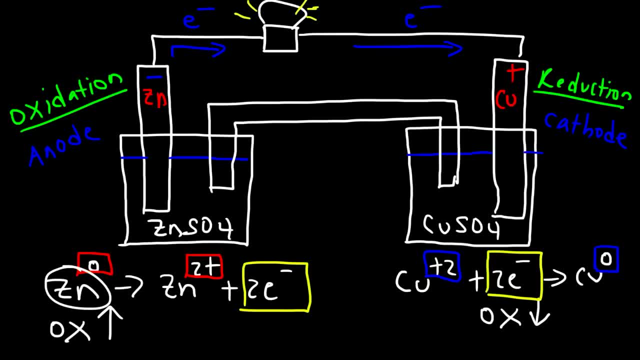 the anode. Now, as the zinc atoms lose electrons, they turn into zinc ions. So let's say this is a zinc atom here. It's hard to see it, but let me just redraw it like this. So when that zinc atom gives up two electrons, it's going to 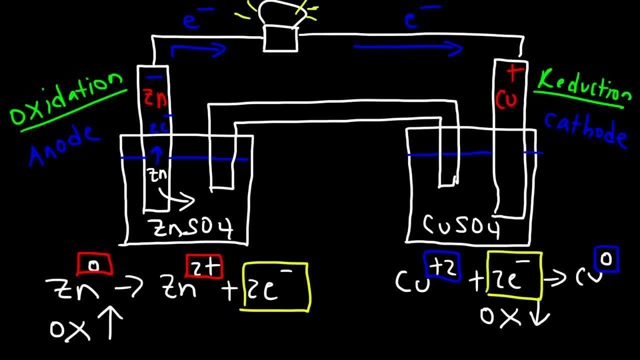 turn into an ion And so it leaves the electrode and it dissolves in a solution. Now on the other side there's already copper ions in a solution. So a copper ion is going to be attracted to the incoming electrons because opposite charges attract, As the electrons flow on this metal into the solution, well, they. 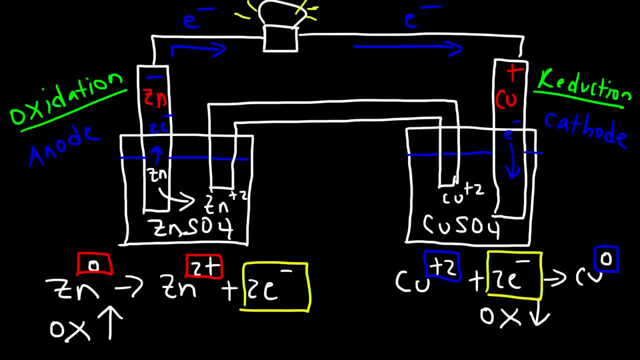 don't really flow into the solution, but they're flowing through the metal in the direction of the solution. these copper ions, they're attracted to the negatively charged electrons And so they're going to accelerate towards that electrode. And as they accelerate towards the 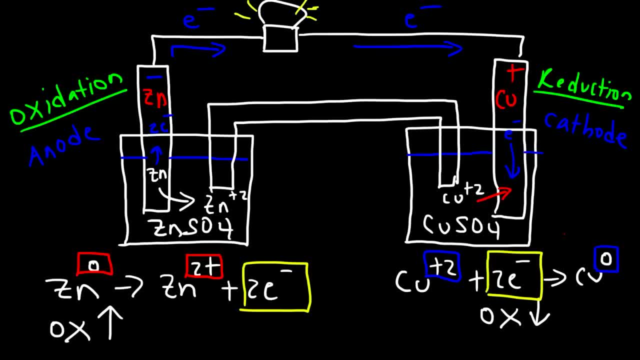 cathode. they're going to pick up the electrons at the interface between the cathode and the solution, And so, as these ions acquire electrons, they turn into copper metal And so they deposit themselves on the surface of the cathode. So over time you'll notice that the cathode is going to get bigger. 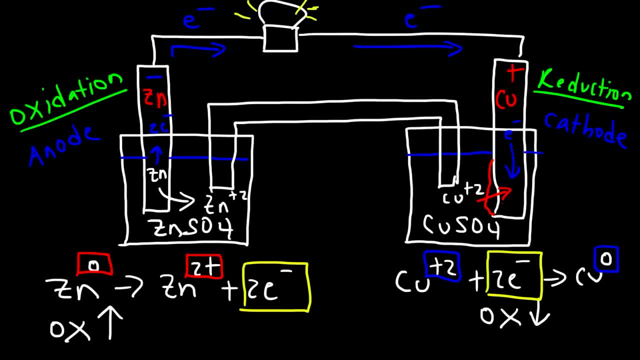 because the copper ions are turning into copper atoms on the surface of the copper electrode. Now the zinc electrode is going to get smaller Because it's losing mass. So in a galvanic cell, the anode, it loses mass, The cathode gains mass. So as electrons flow from anode to cathode, the anode is. 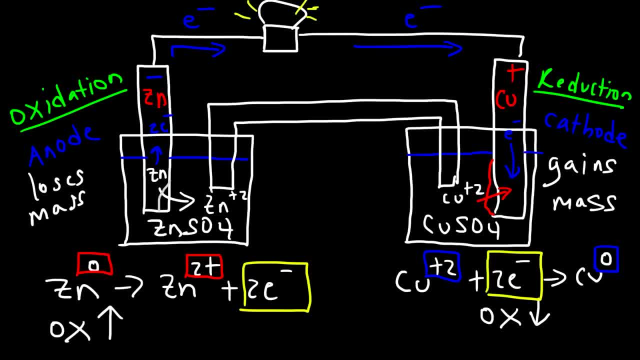 going to lose mass and the cathode is going to gain mass. Make sure you understand that. So this electrode is going to slowly disappear and this one is just going to get bigger. And that's the basic principle for electroplating: You can transfer mass. 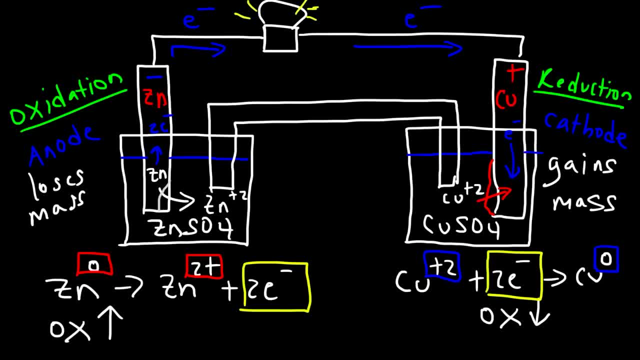 from one electrode to another electrode, but we'll talk about that in another video. Now there's another element that we need to talk about, and that is the cell bridge. What do you think is the purpose of the cell bridge? Why do we need it? Without the cell bridge, current will flow only for a very 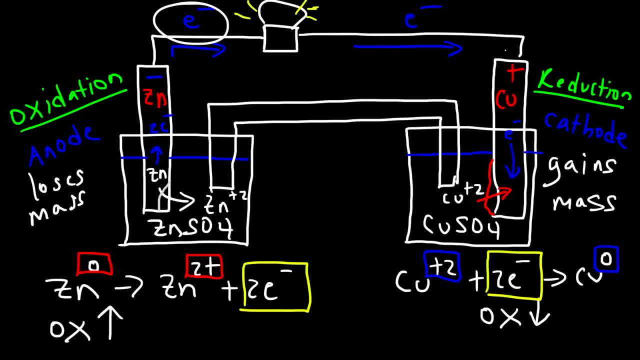 short time. You're going to have some electrons flow from the anode to the cathode, but as electrons flow towards the cathode, this side is going to have a buildup of negative charge and this side is going to have a buildup of positive. 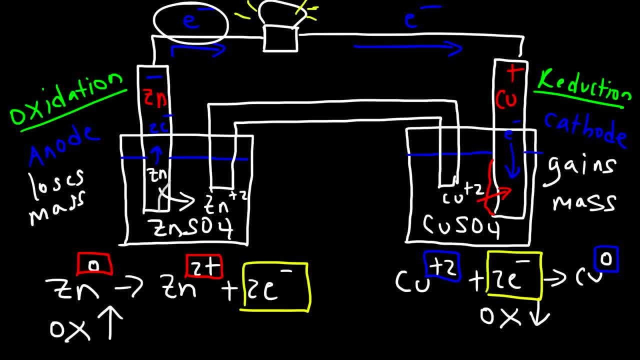 charge because it lost electrons, And so once you have that charge, buildup electrons will no longer flow, Because once this side becomes positively charged, the electrons that went this way is now attracted to this side, And so it's going to reach a state of equilibrium, And so without the salt, 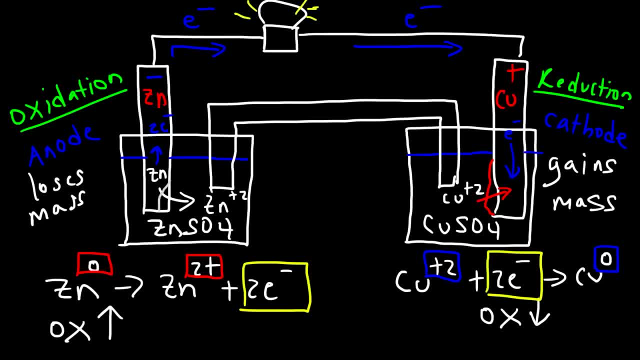 bridge, you won't have a constant flow of electricity. It's going to be very short-lived, And so the purpose of the salt bridge is to keep the solutions neutral, So as electrons flow from anode to cathode, this solution becomes negatively charged. 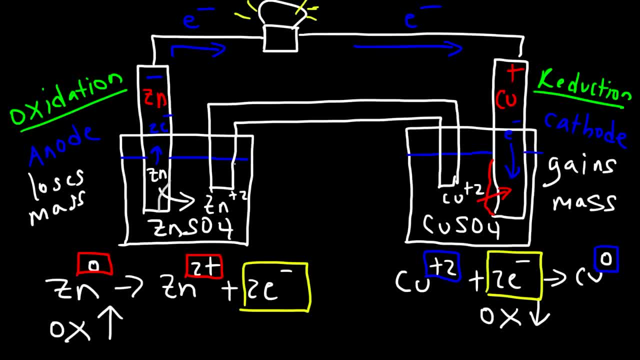 This becomes positively charged. So to relieve the positively charged nature of this solution, what happens is the anions which are known as positively charged ions, they're going to flow through the salt bridge to the other solution. So the zinc cations are going to flow towards the cathode Cations. cathode makes sense. 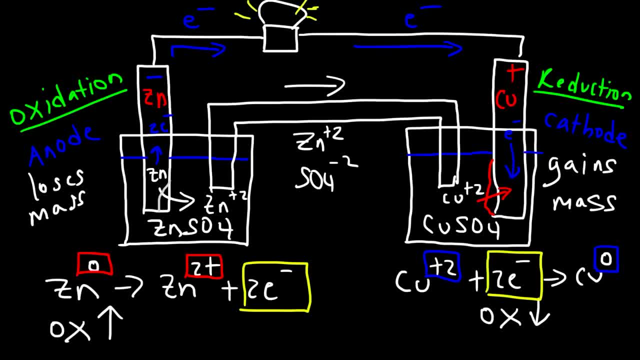 The anions flows toward the anodes. Now, this works in such a way that the two solutions remain neutral, But keep that in mind. Anions flow towards the anode, anions are negatively charged particles, and cations flow towards the cathode, And so that's how the salt bridge will prevent. 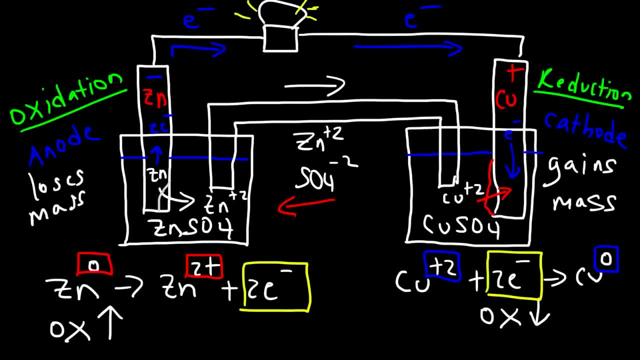 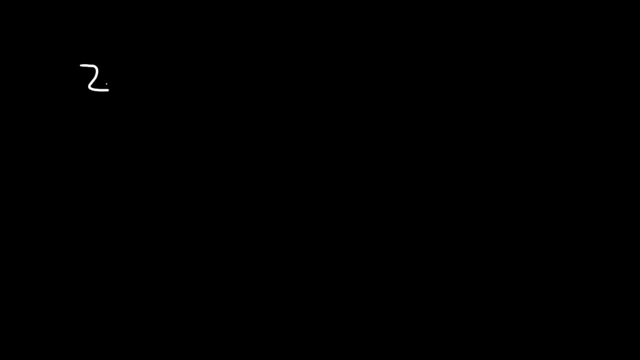 a buildup of charge. So now that we've discussed the basic operation of a galvanic cell and how it works, let's talk about the cell potential and how to calculate it for this overall reaction. So we saw that zinc turns into the zinc 2 plus ion by giving up two 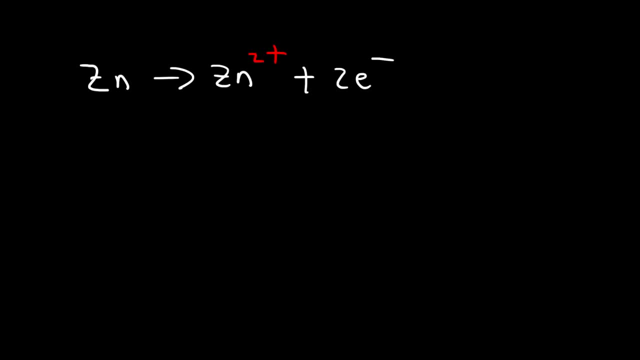 electrons. Now the cell potential for this half reaction is positive, 0.76 volts, And so this occurs at the anode. I'm going to write A for anode, And so that's the oxidation half reaction. So remember, anytime you see the 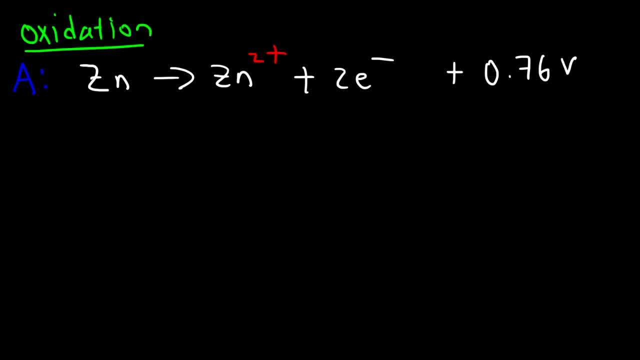 electrons on the right side, it's oxidation. If the electrons are on the left side, it's reduction. Now the other half reaction. the copper 2 plus ions acquire electrons and turn into copper metal, And the cell potential for this half reaction is positive 0.34 volts. So this: 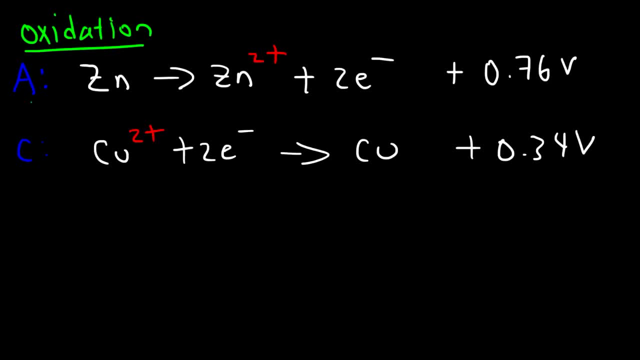 occurs at the cathode And reduction always occurs at the cathode. So anytime you see the electrons on the left side of a half reaction, you know it's associated with a reduction half reaction. So we can do is add up these two half reactions. Notice that we have two electrons on the left and two. 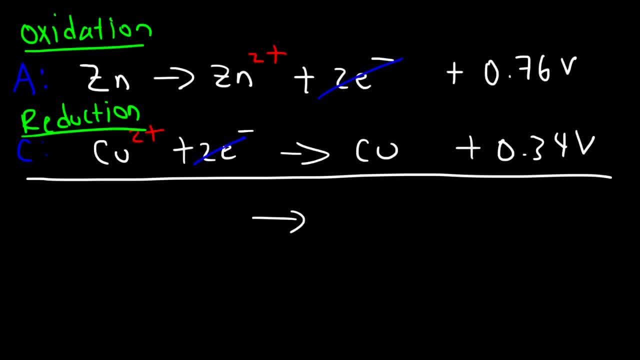 electrons on the right and they will cancel. So on the left of the arrow we have zinc and copper 2+. So this is going to be zinc plus copper, And on the right side we have copper and zinc 2+. So zinc is a metal, so it's in a solid state. 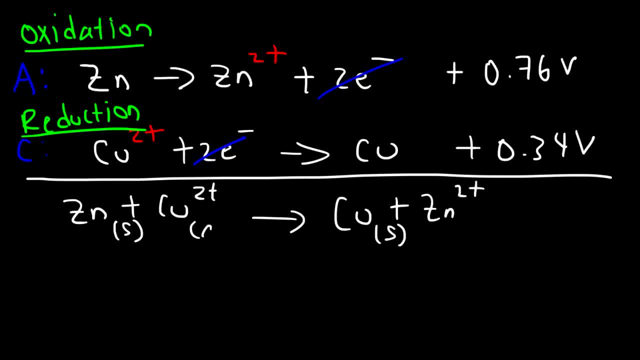 And on the right side, copper is a metal. Now the ions are dissolved in water, so they're in the aqueous state. Now, to calculate the cell potential for this overall reaction, all we need to do is add up these values, So 0.76 plus 0.34 gives us an overall cell potential of 1.1.. 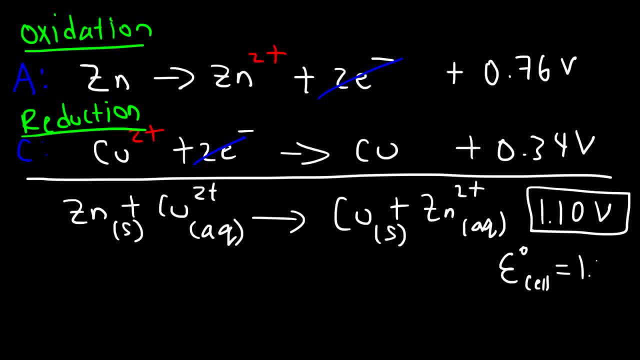 The cell potential looks like this, So it's 1.1 volts. Now we can represent the cell using a line notation or a cell notation. So first you need to write the anode, which is zinc, And then use a single vertical line to separate the phases, because these two phases are different. 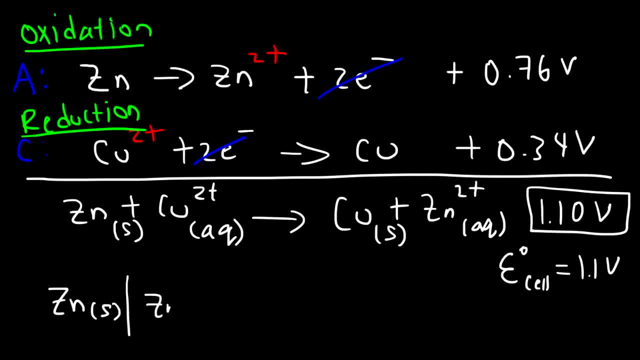 So in the solution we have the zinc 2 plus ion, That's in the first compartment on the left, And then you need a double arrow to separate the anode half cell from the carbon, And then you need a double arrow to separate the anode half cell from the carbon. 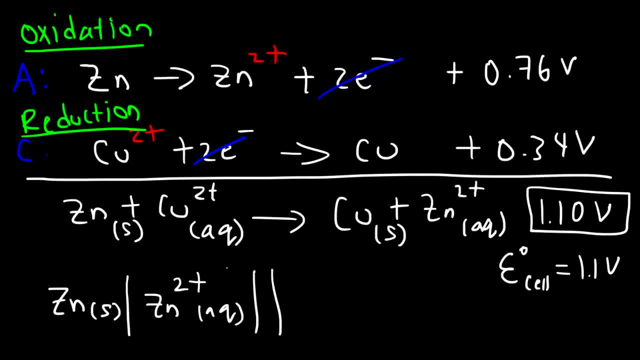 And then you need a double arrow to separate the anode half cell from the carbon. So on the left side this is for oxidation, which is associated with the anode, And the right side will be associated with reduction, which is with the cathode. 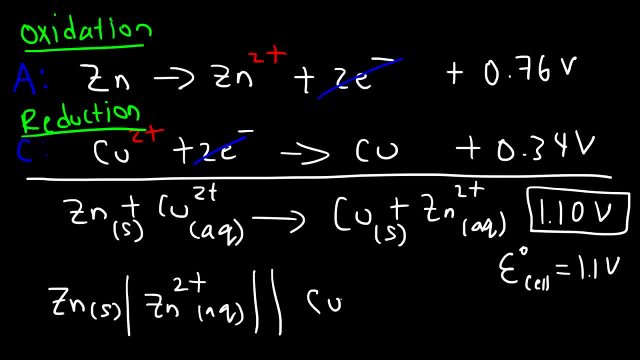 So in the reduction half cell we have the copper 2 plus ion dissolved in the solution, And we need to separate that, because the electrode is in a different phase than the copper 2 plus ion, And so the cathode is copper metal. 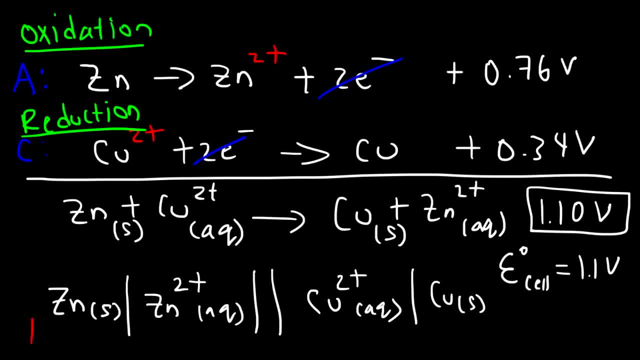 And the anode is zinc metal. So that's a simple way in which you can represent this cell using cell notation, or also known as line notation. By the way, a galvanic cell is also known as a voltaic cell, So just keep that in mind. 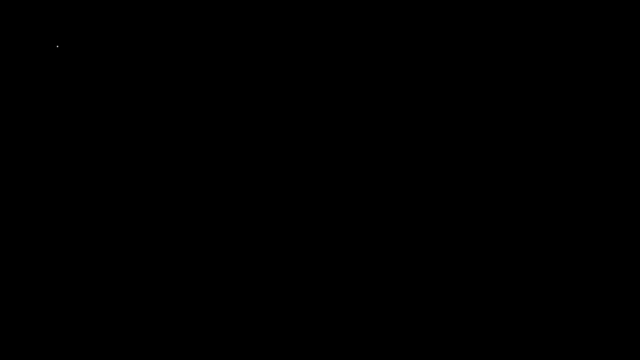 Now let's talk about the cell potential, also known as EMF- electromotive force. This is measured in units of volts, Or you could describe it as a voltage. One volt is equal to one joule per coulomb, So what does this mean? 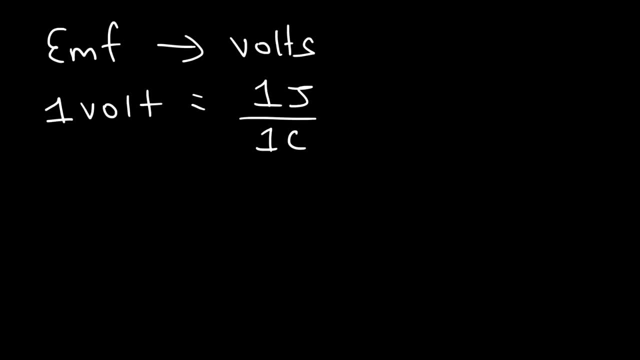 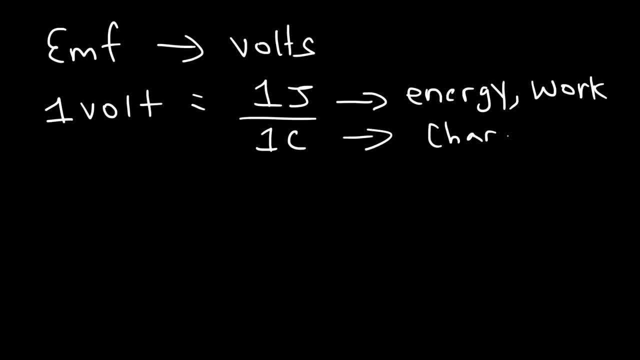 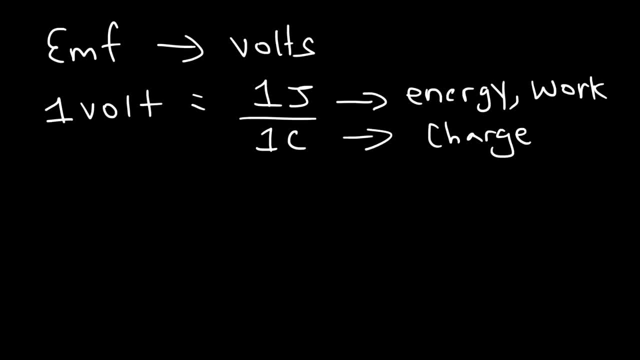 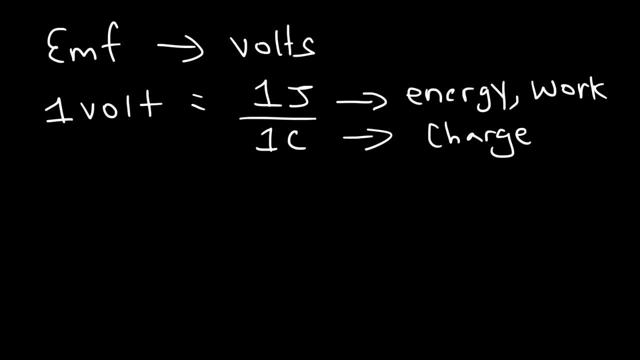 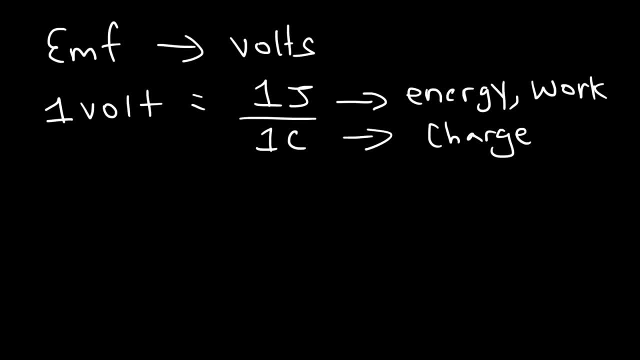 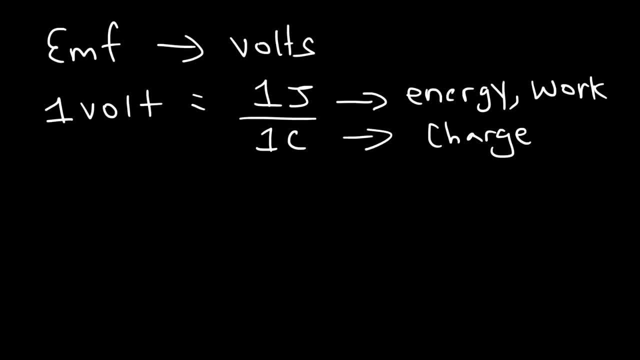 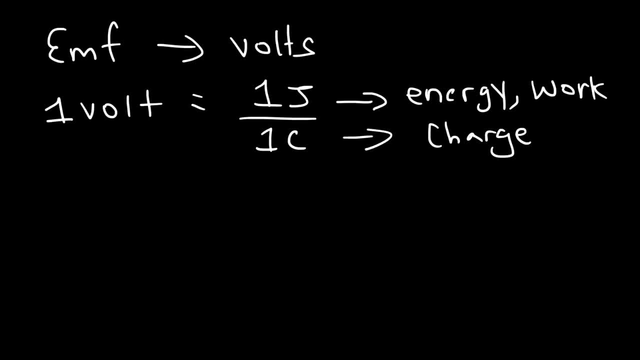 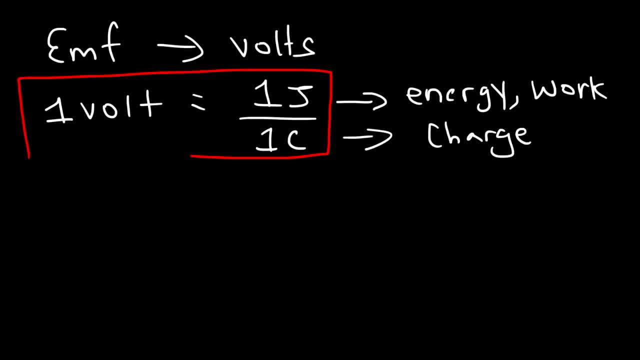 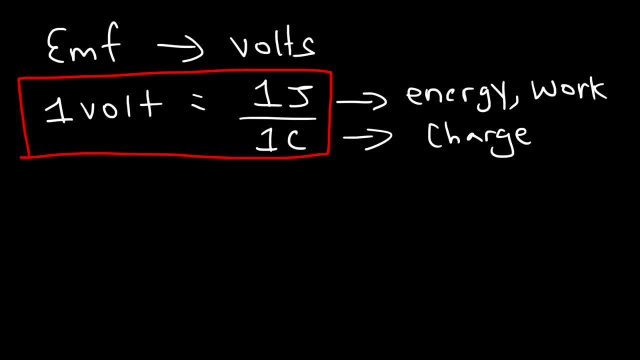 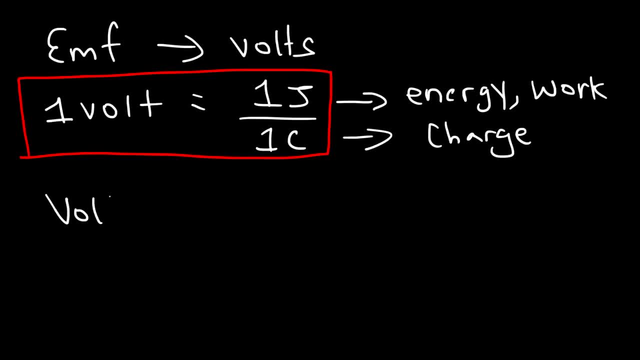 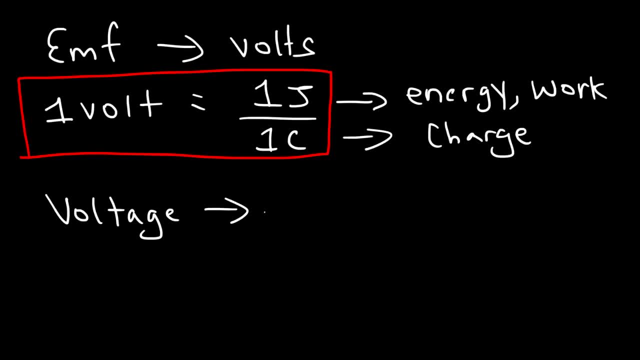 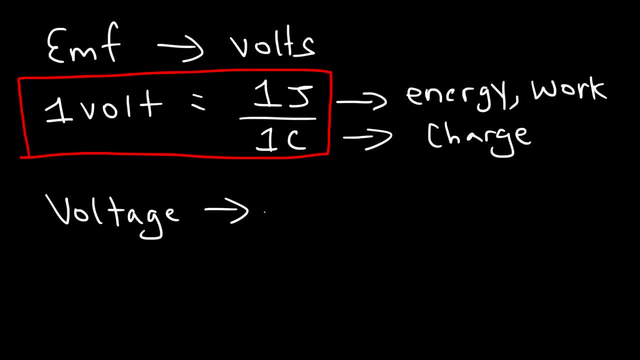 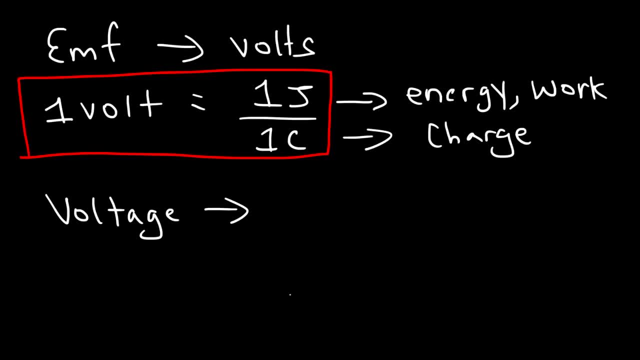 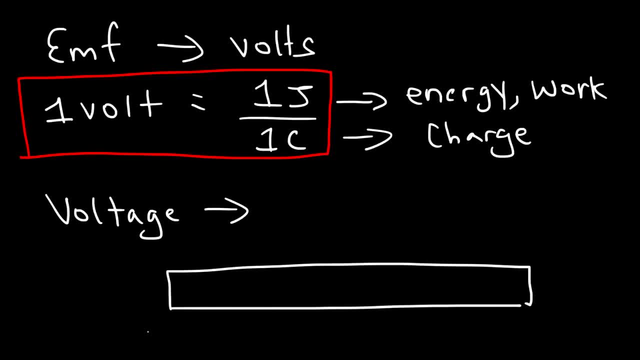 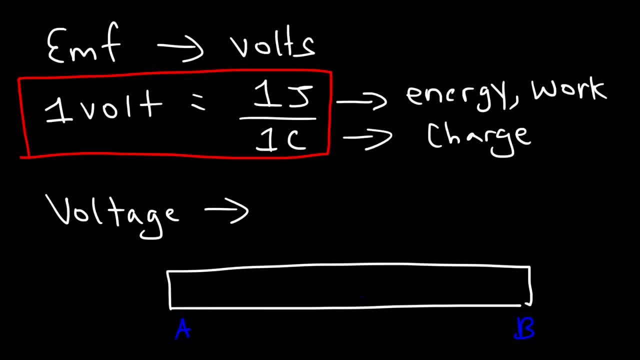 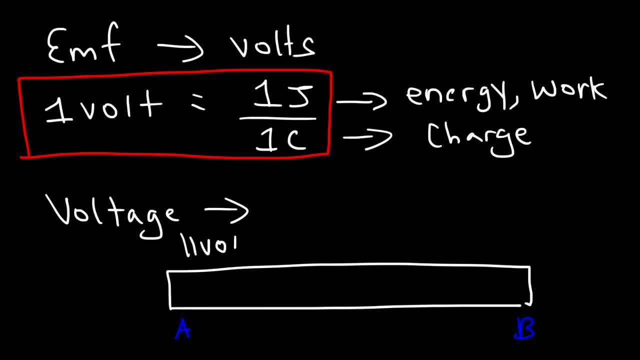 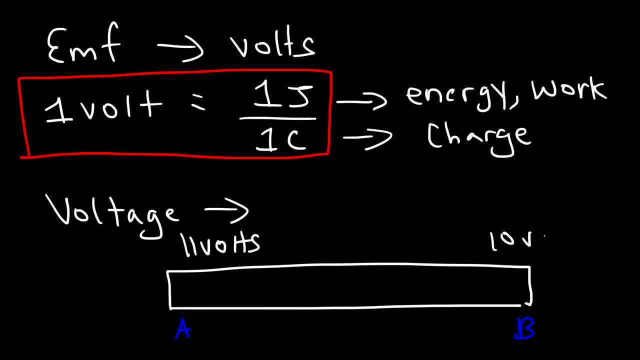 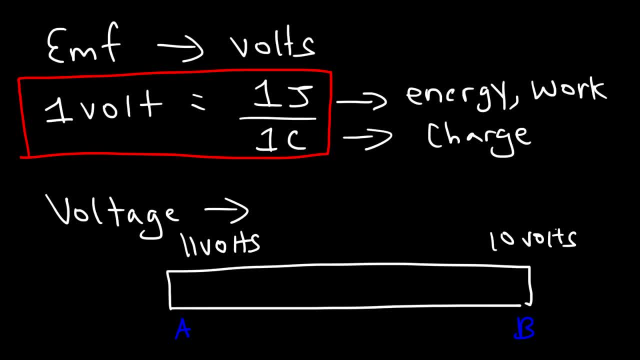 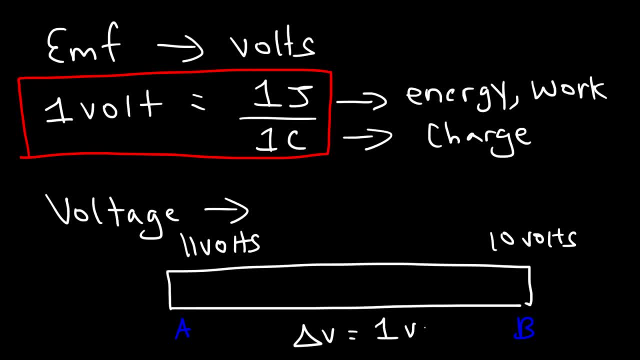 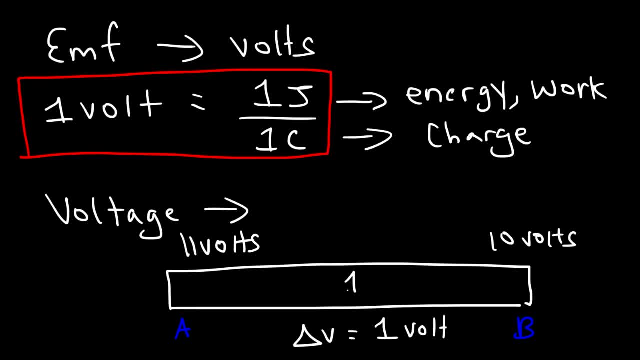 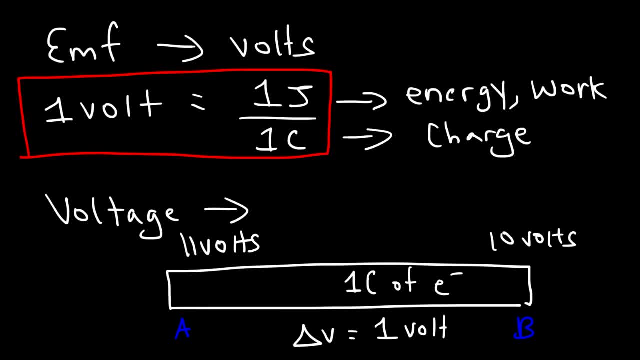 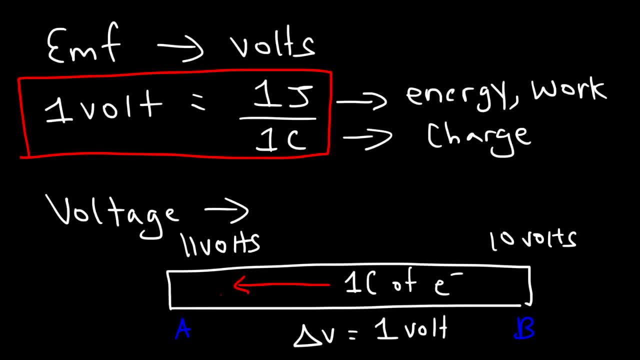 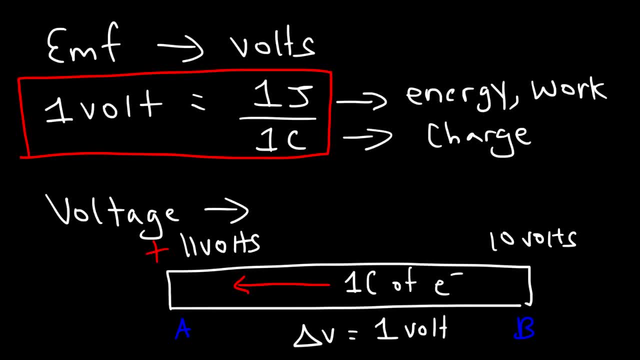 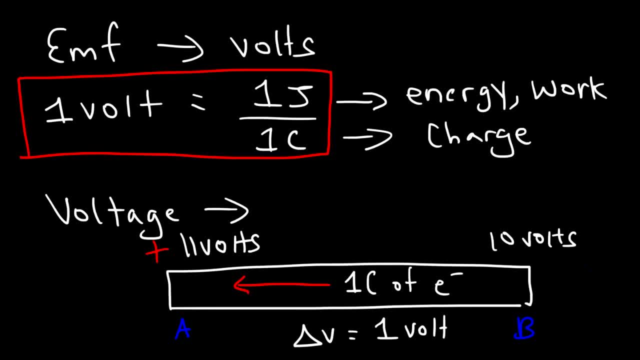 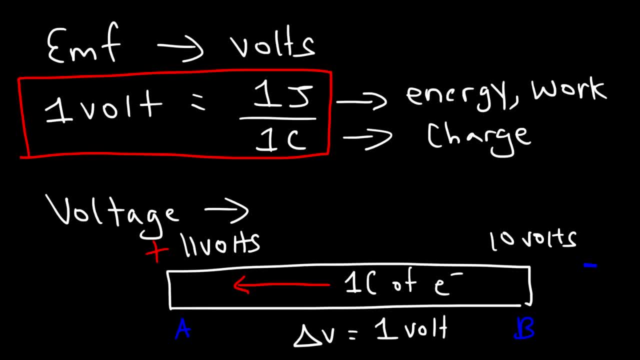 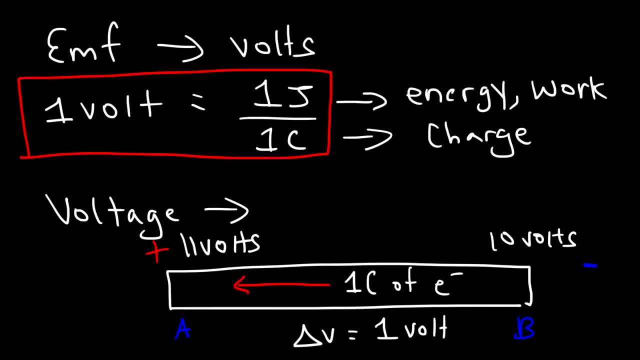 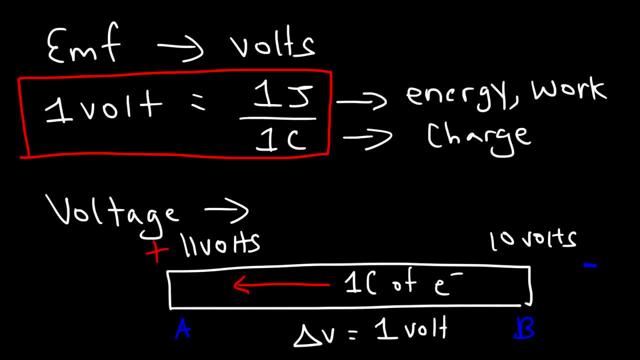 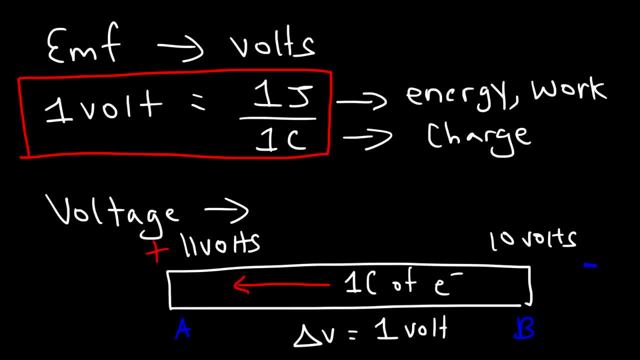 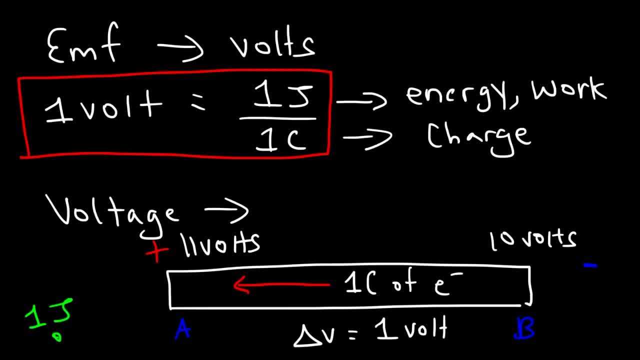 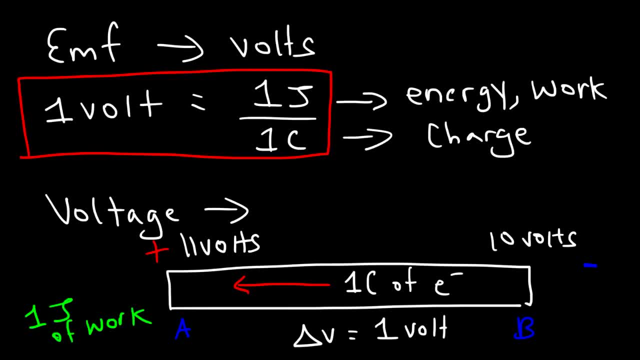 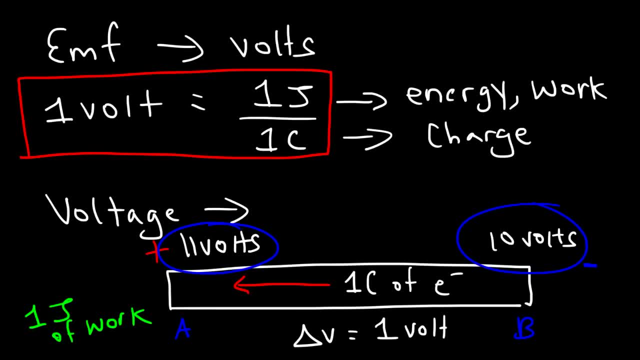 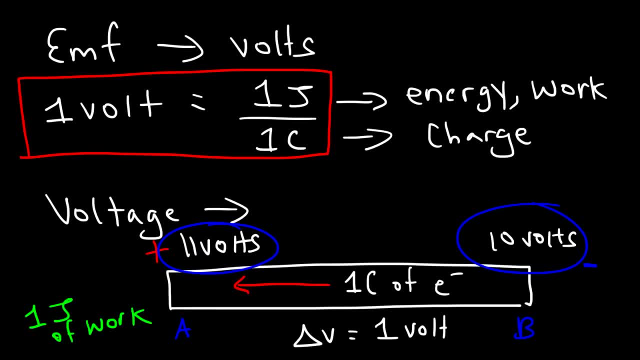 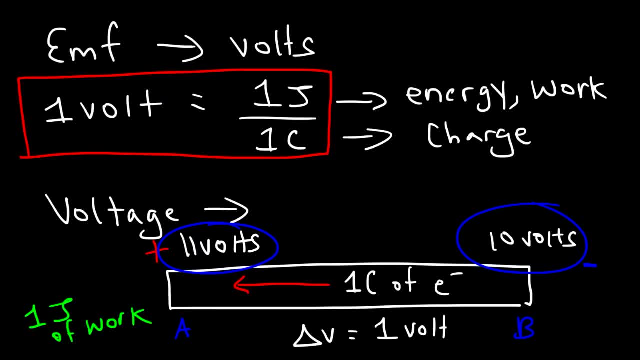 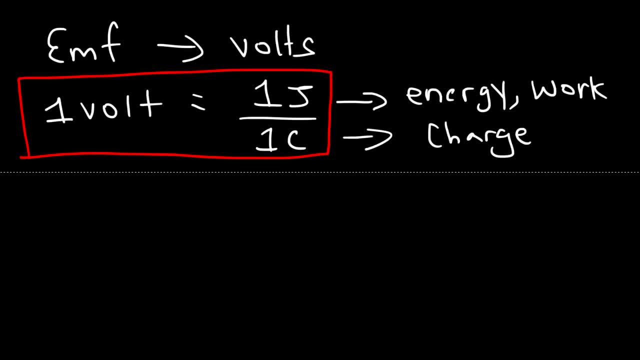 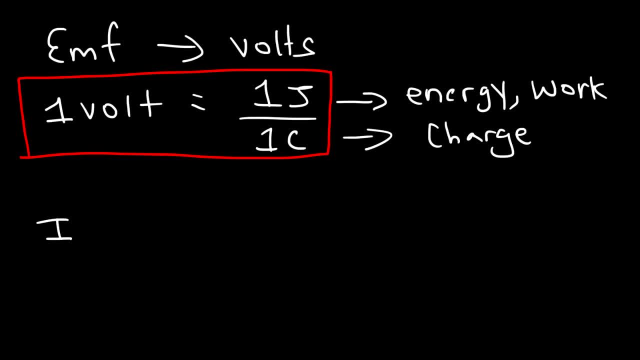 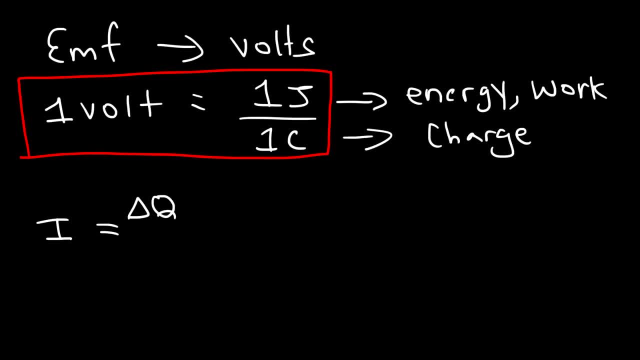 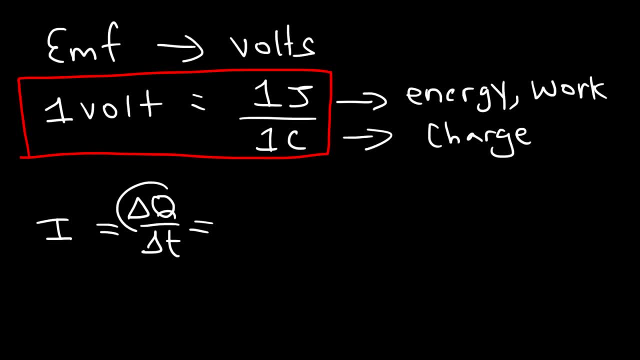 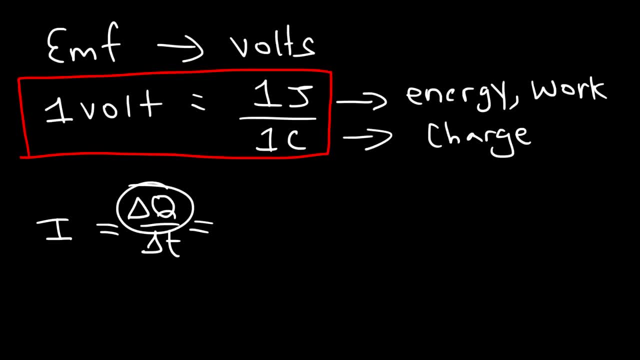 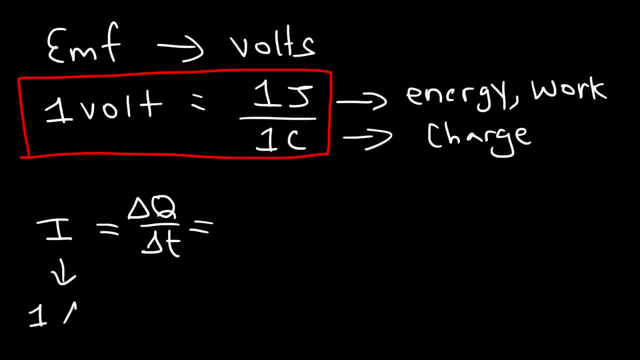 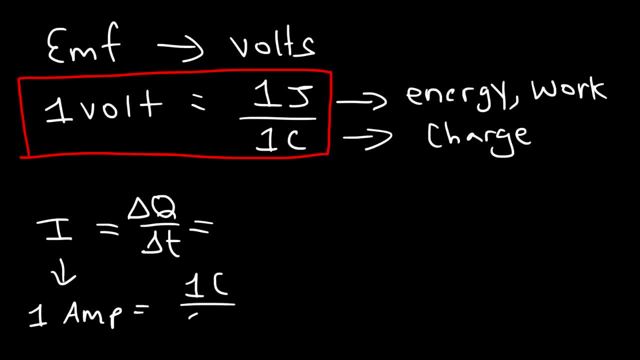 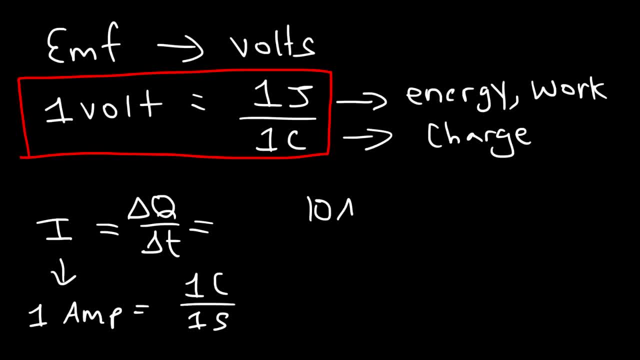 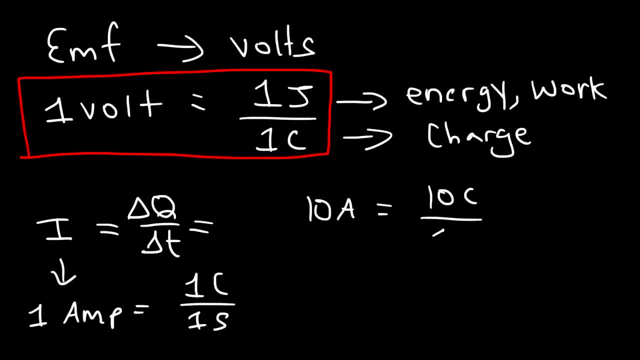 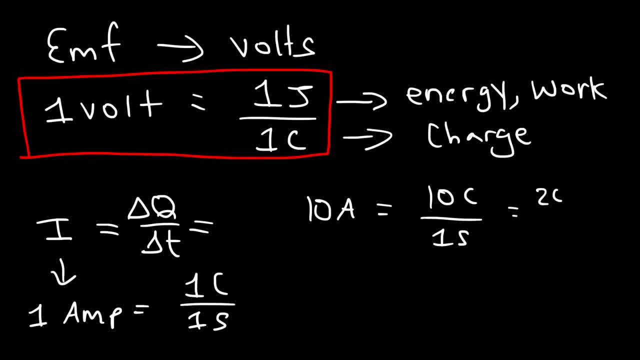 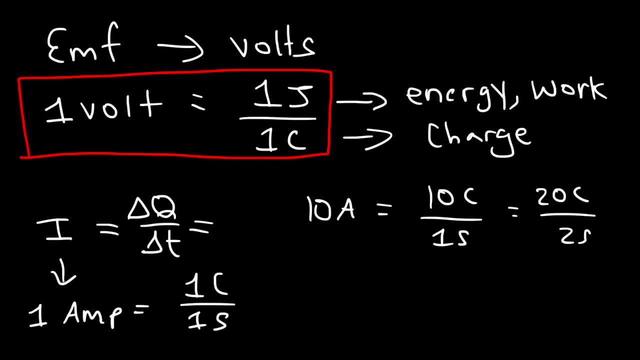 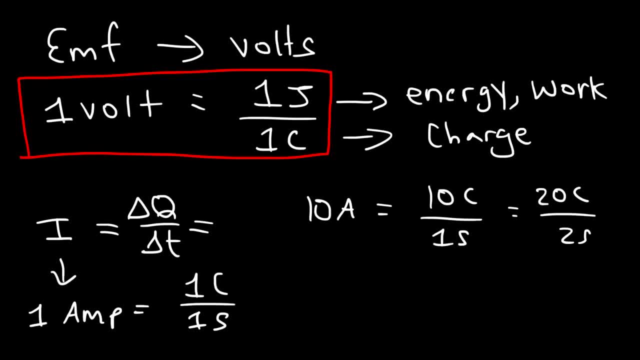 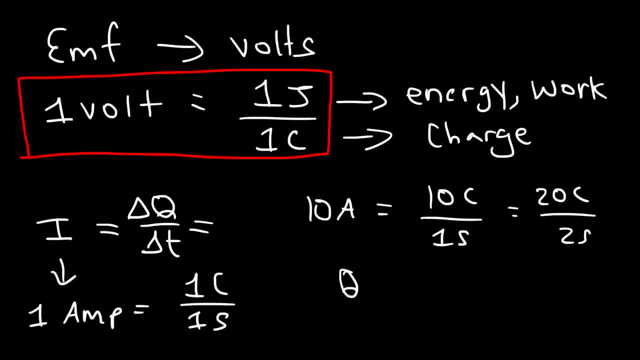 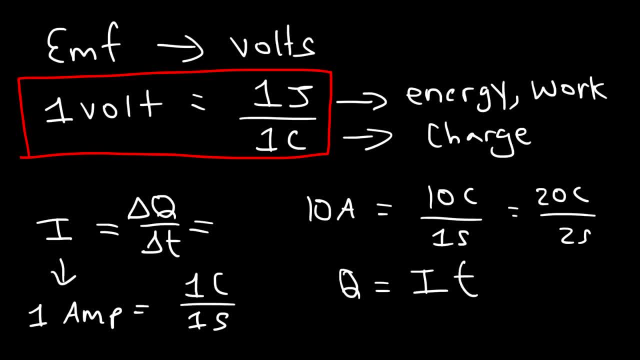 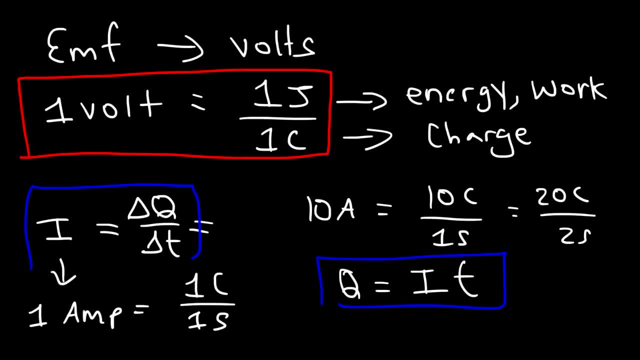 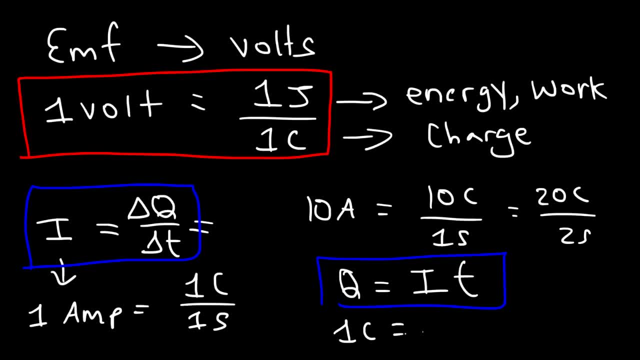 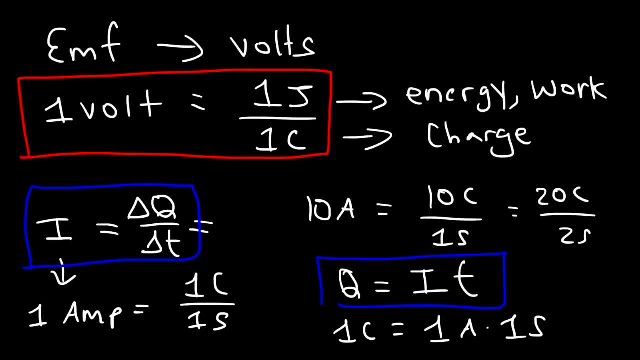 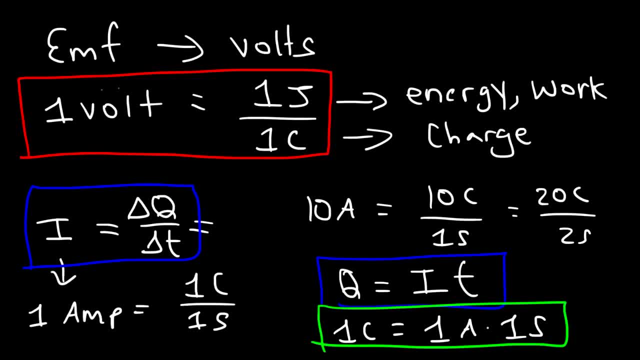 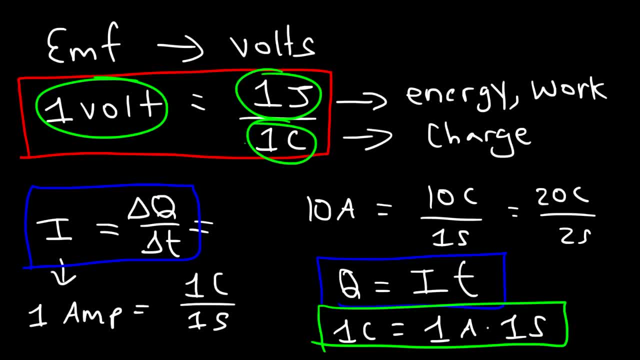 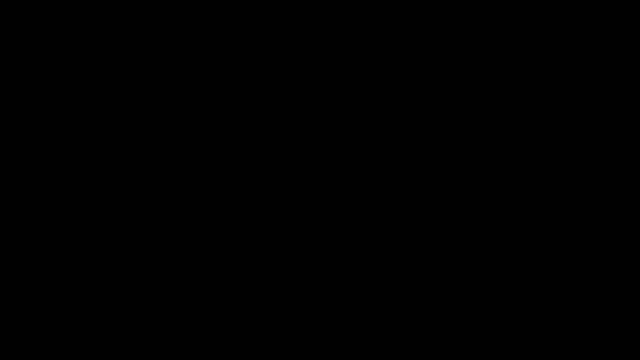 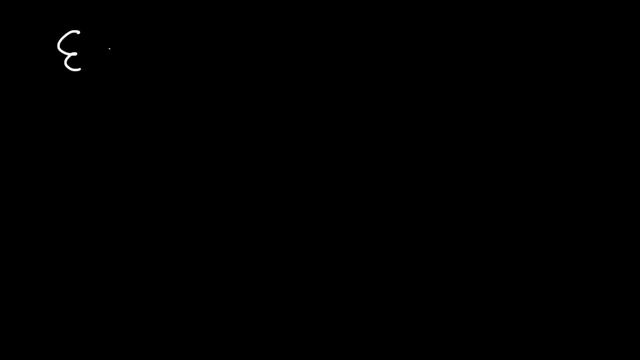 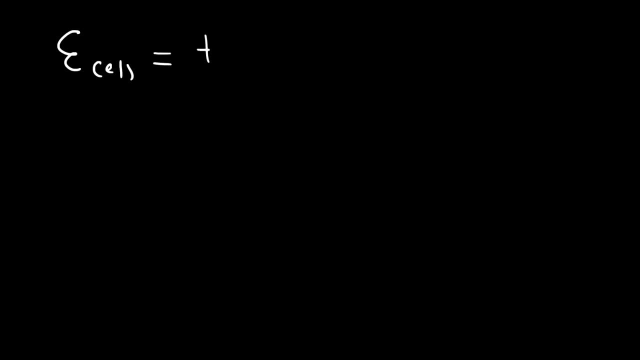 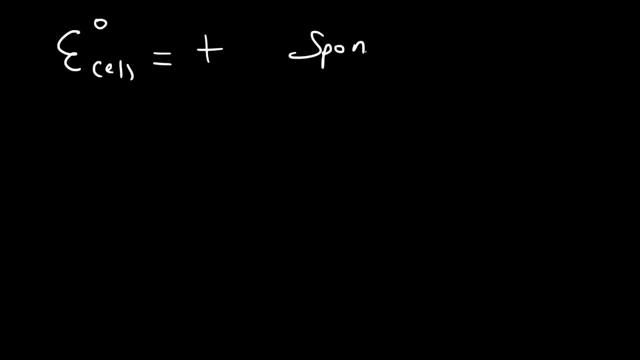 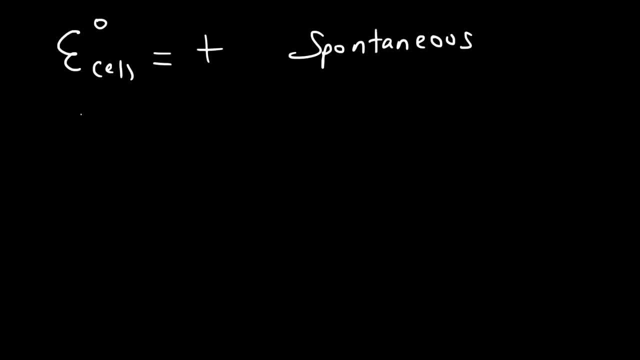 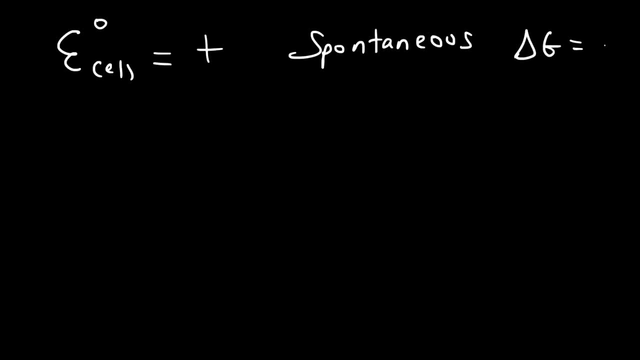 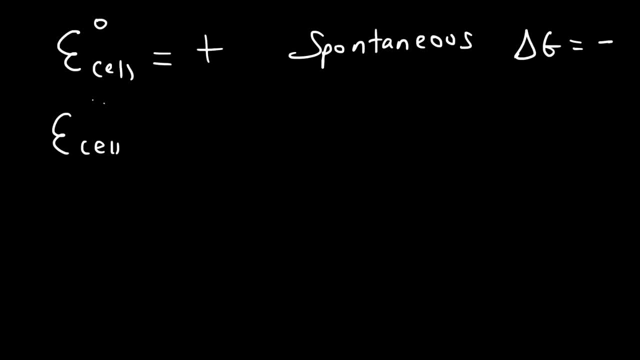 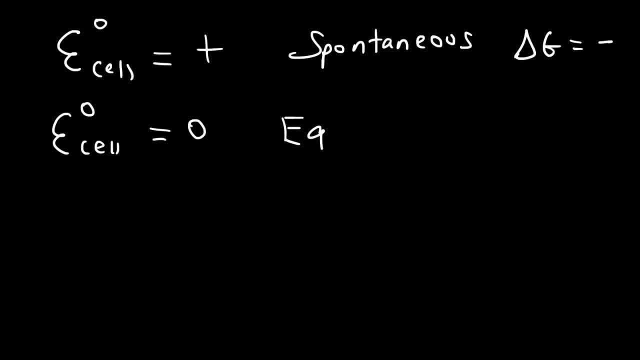 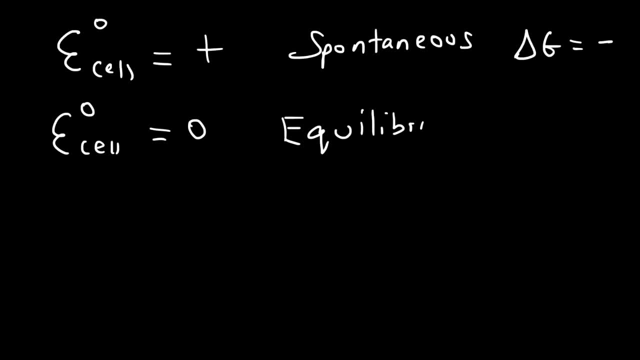 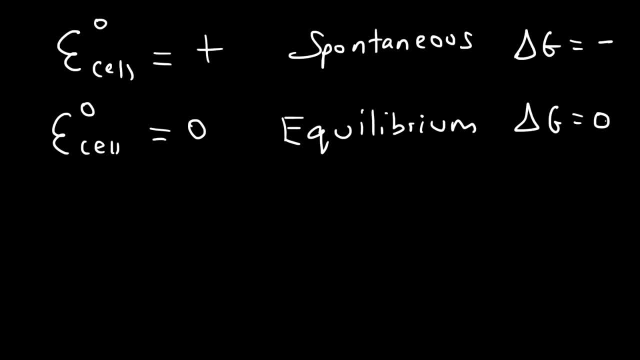 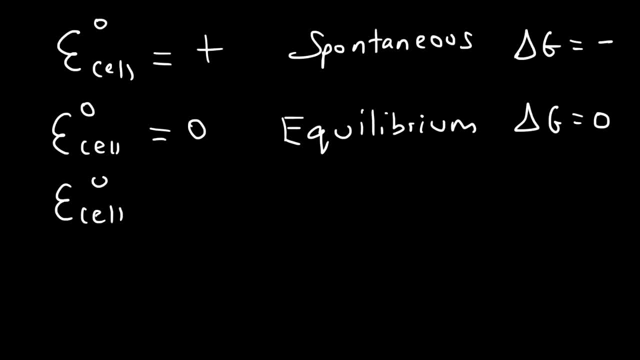 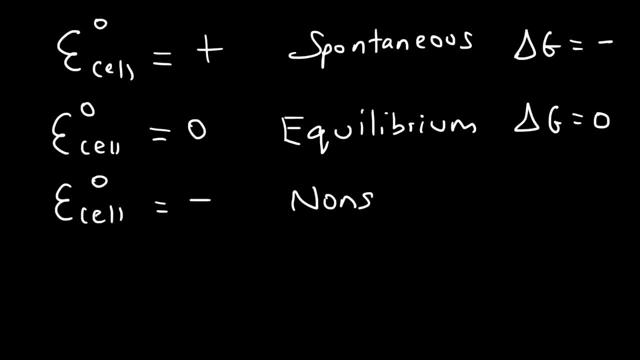 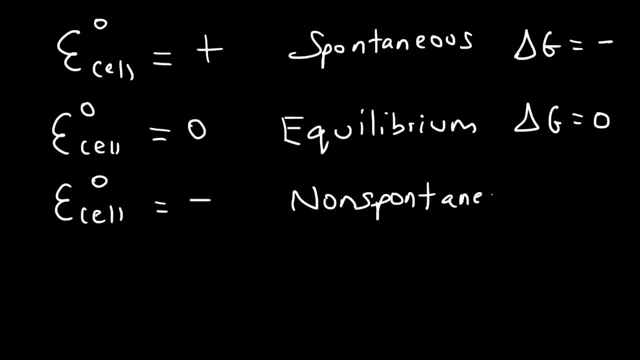 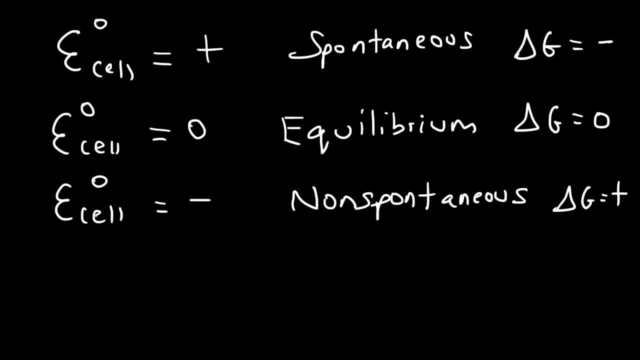 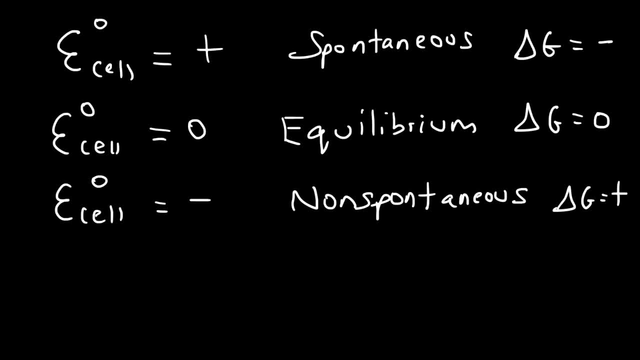 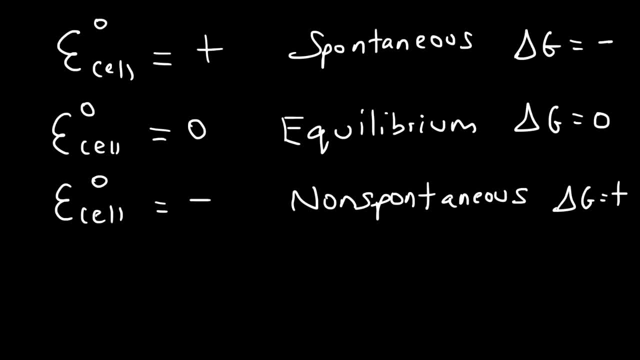 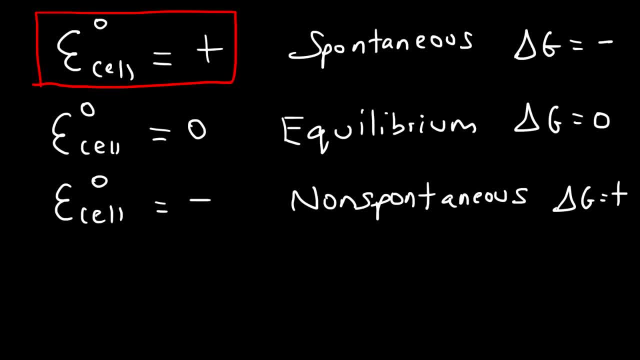 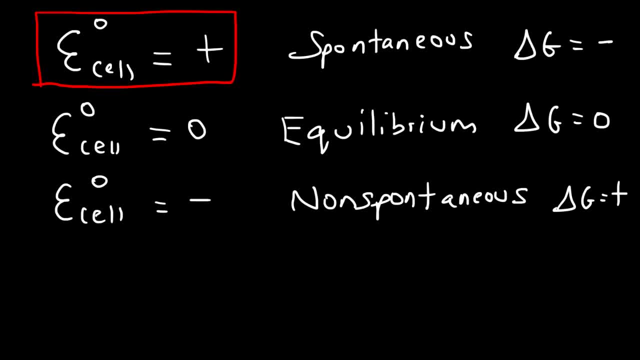 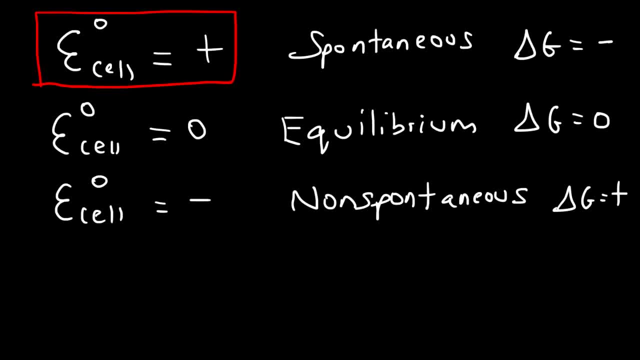 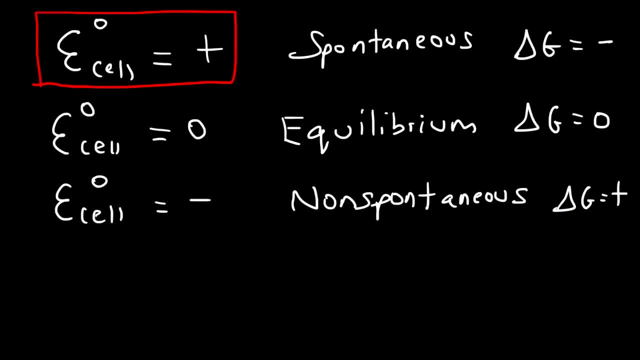 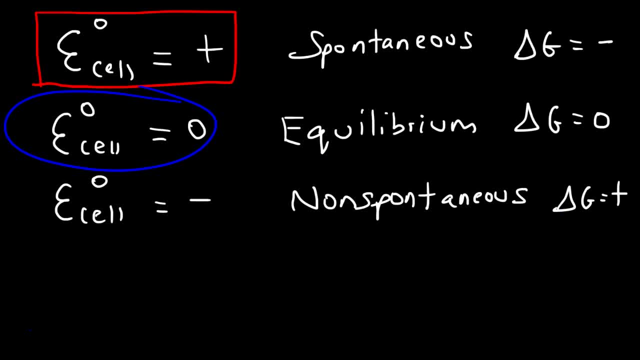 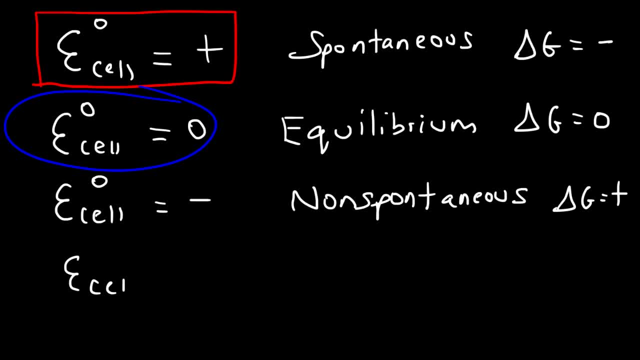 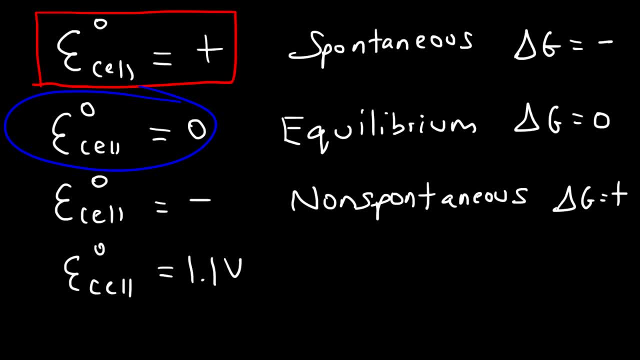 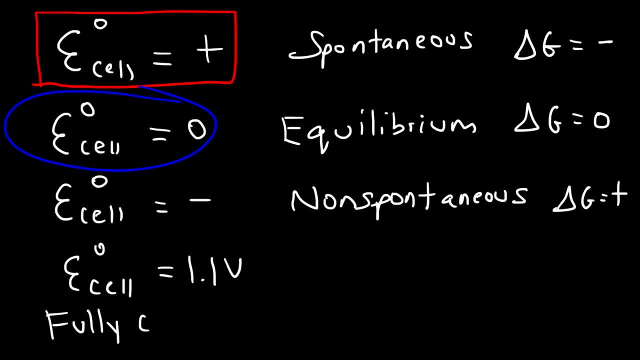 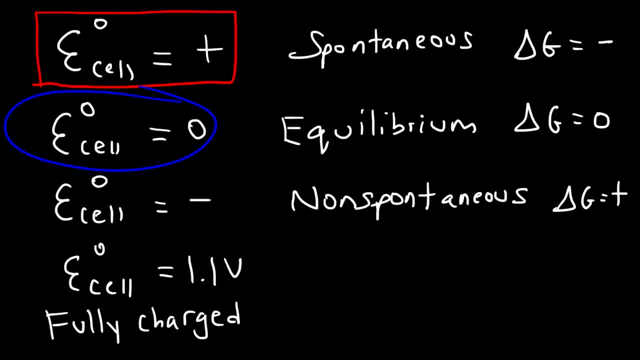 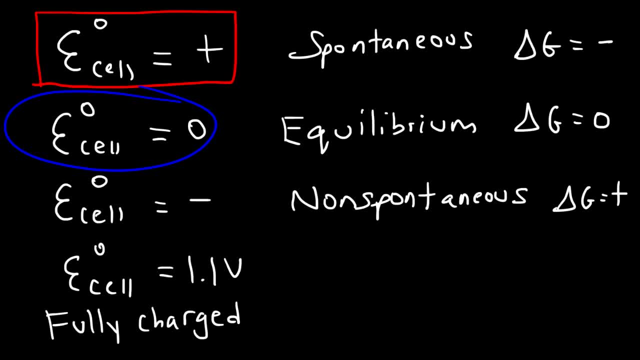 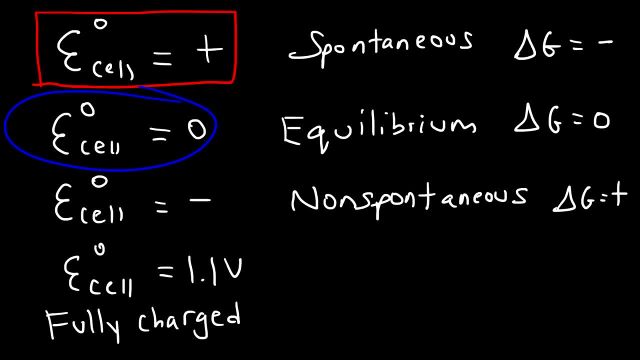 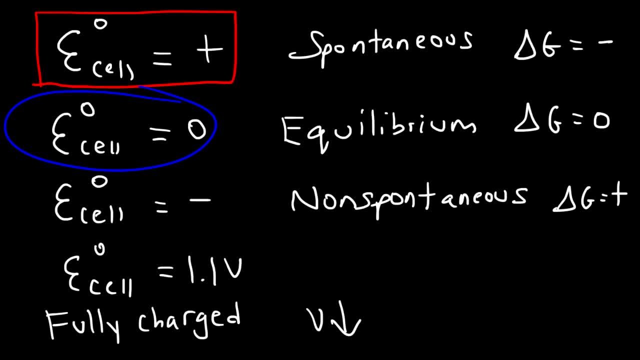 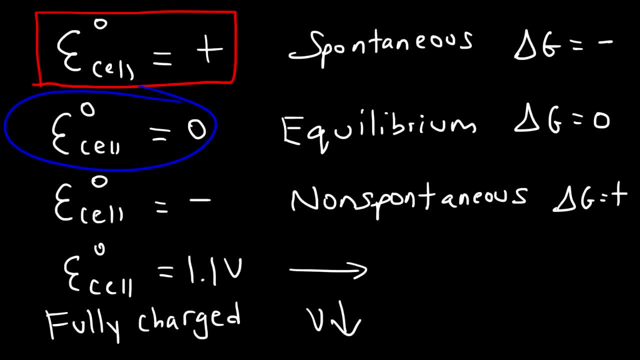 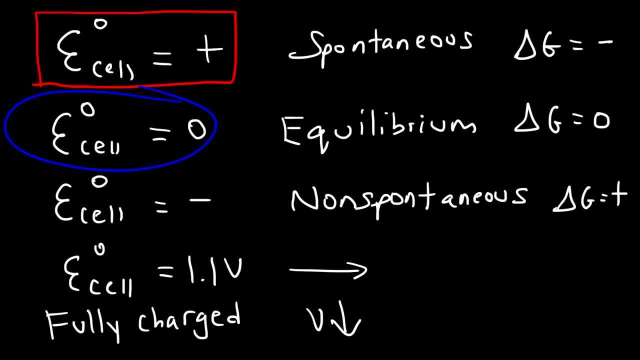 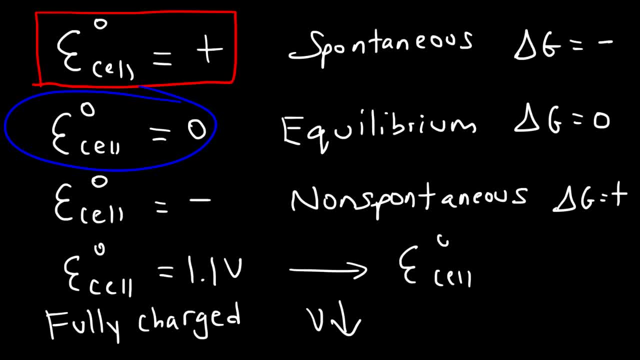 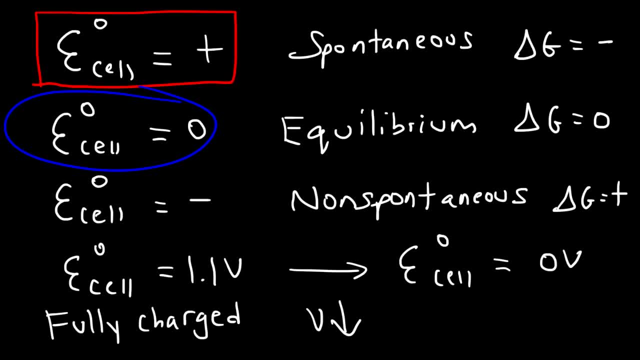 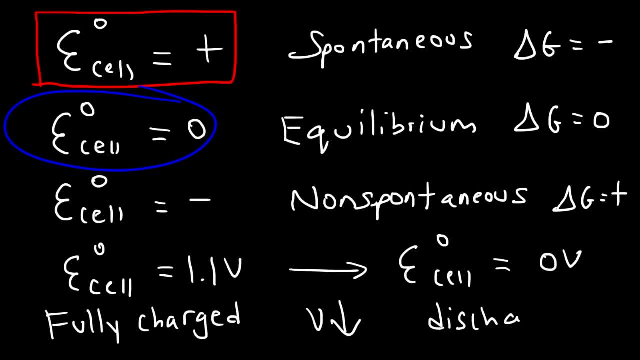 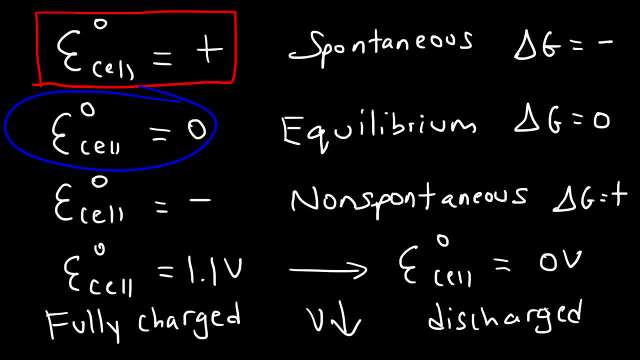 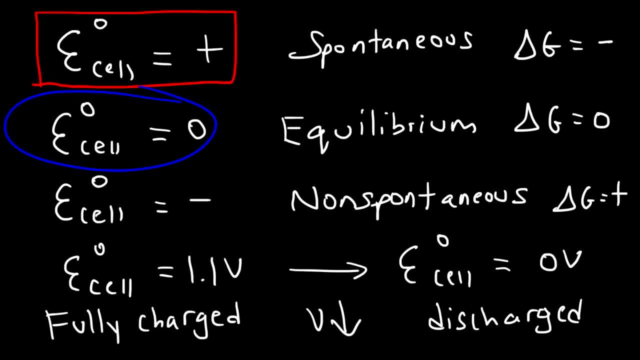 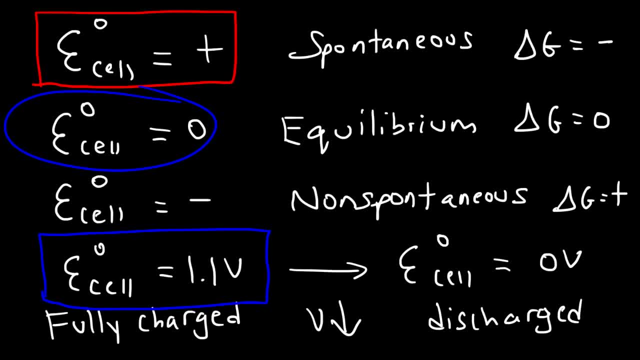 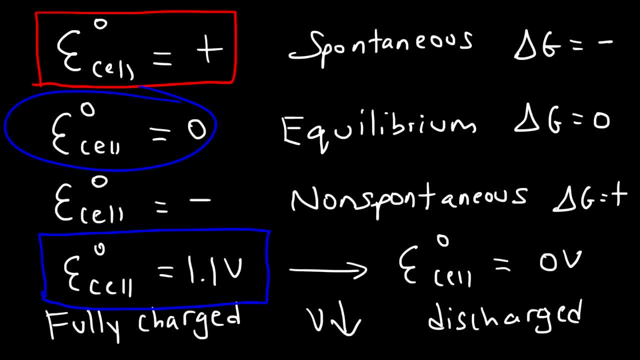 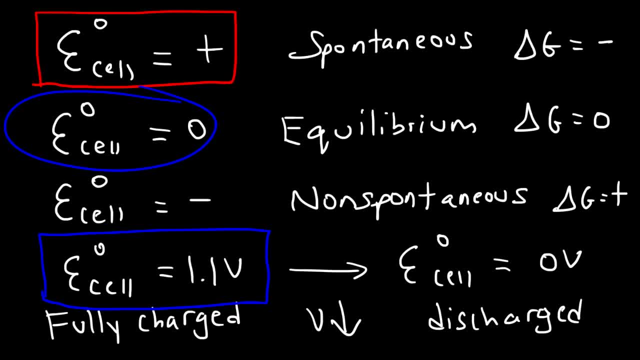 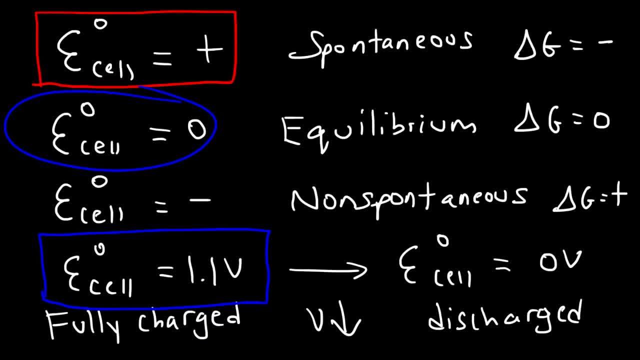 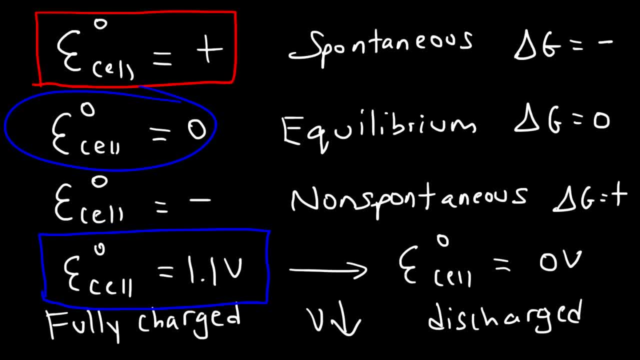 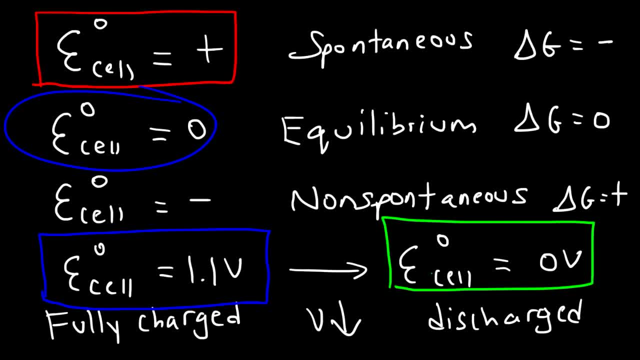 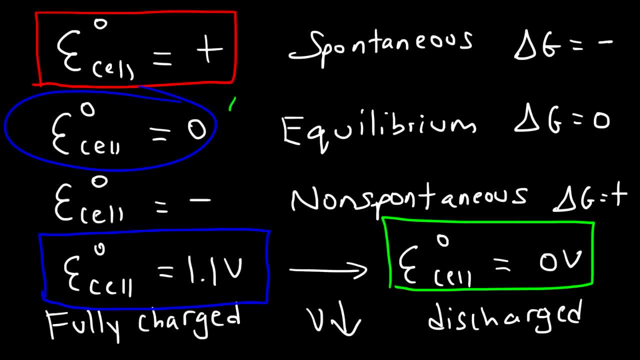 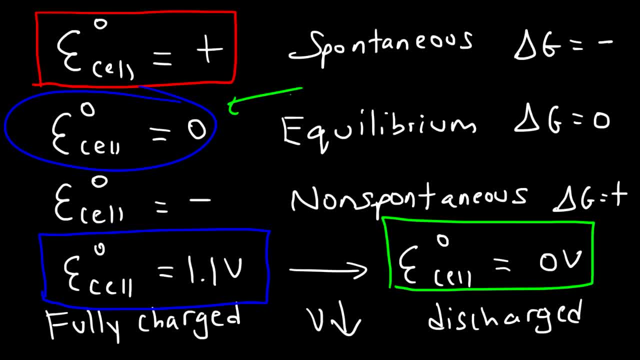 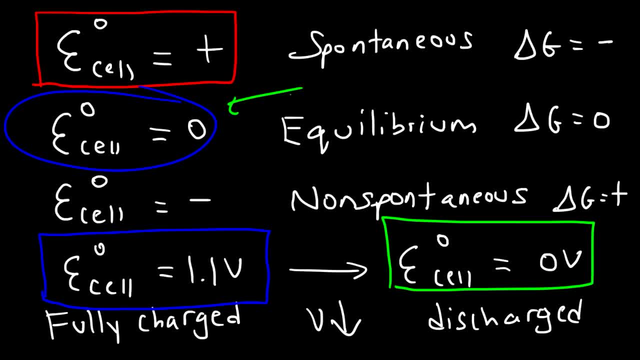 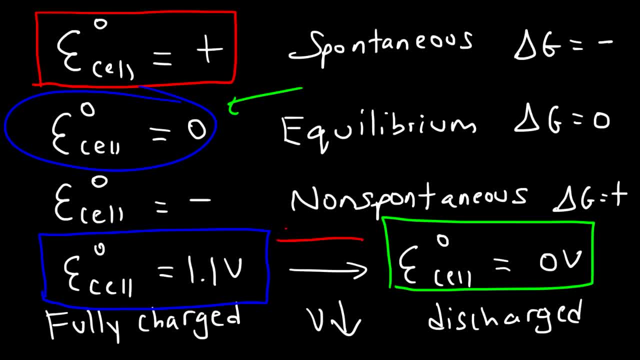 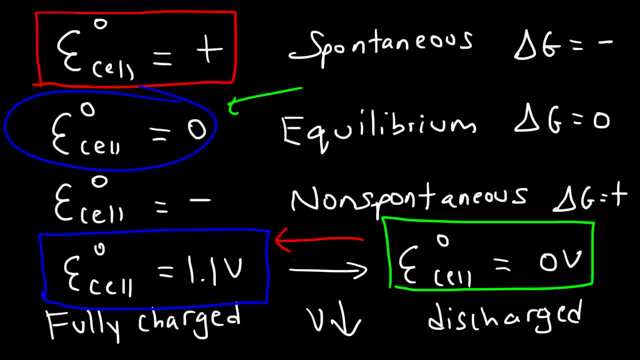 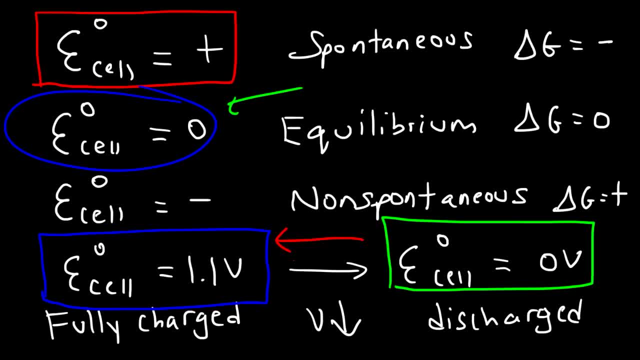 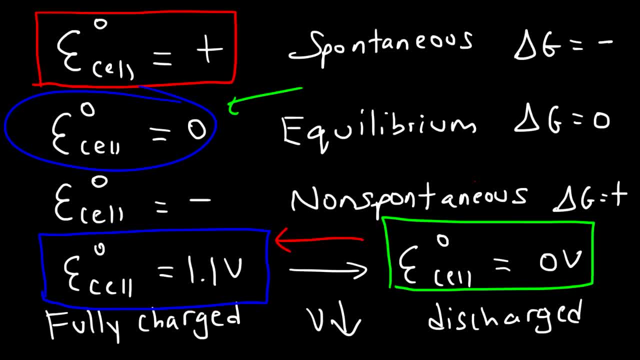 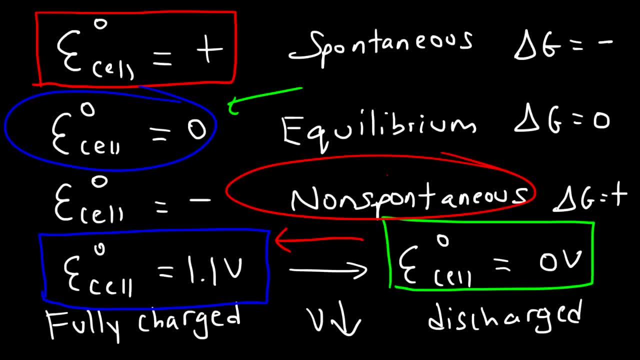 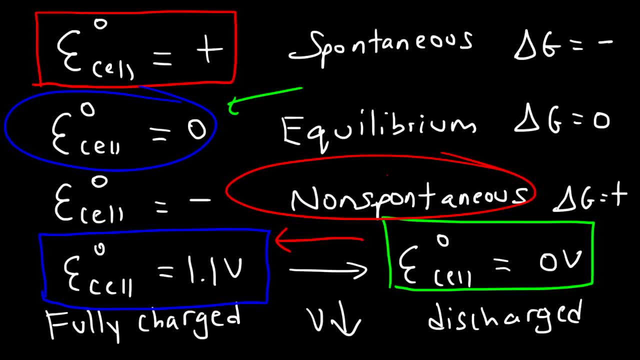 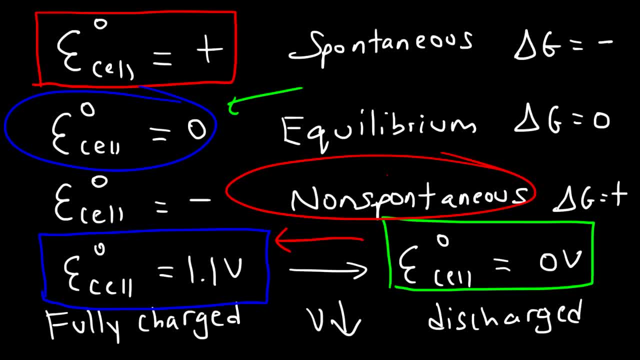 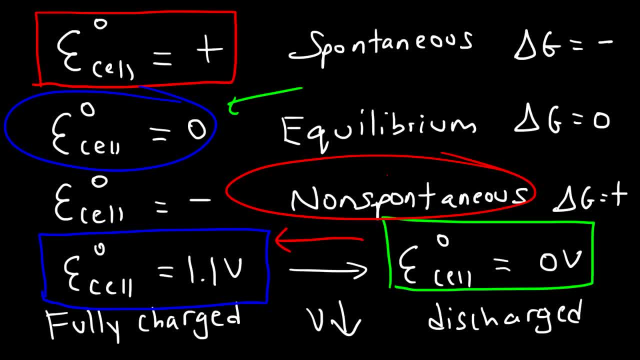 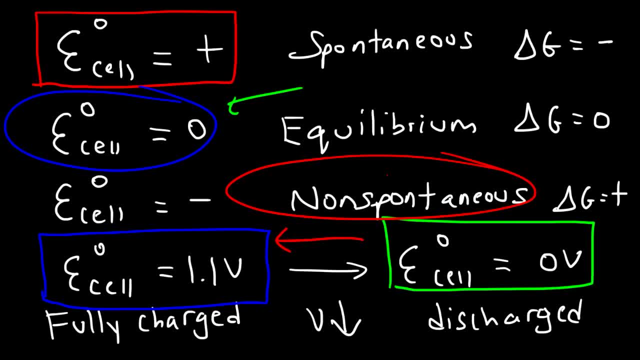 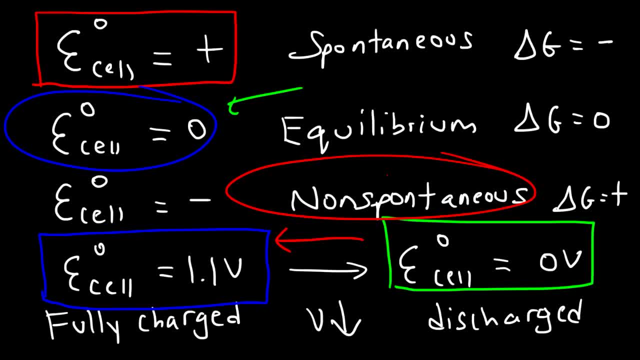 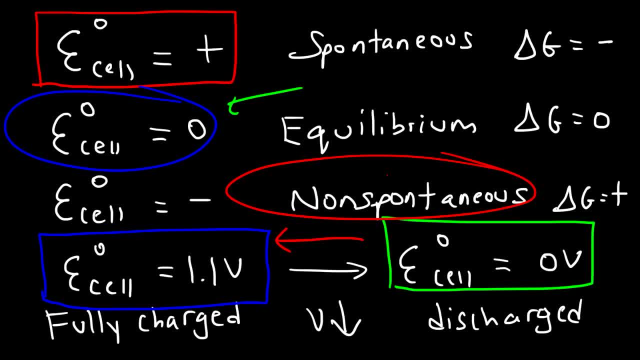 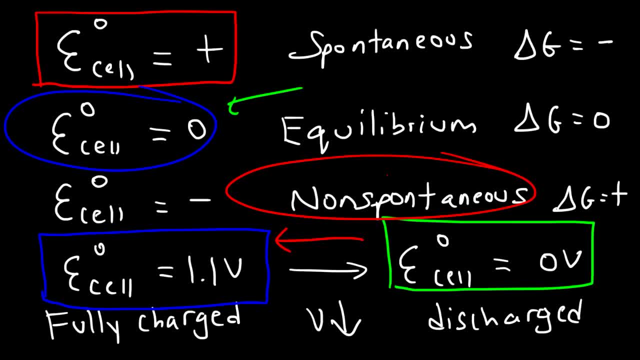 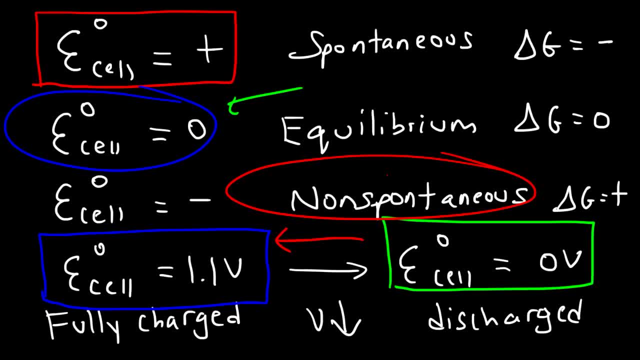 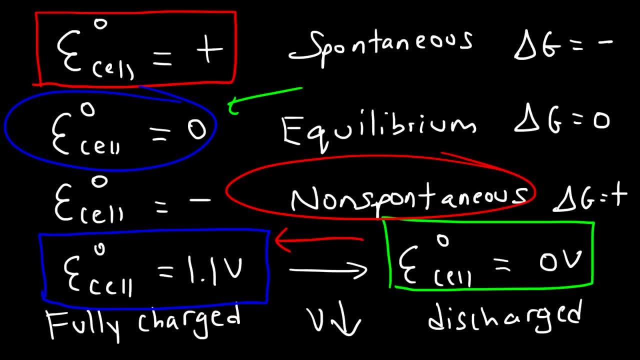 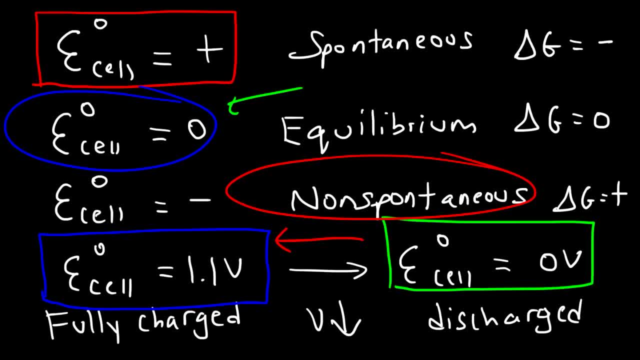 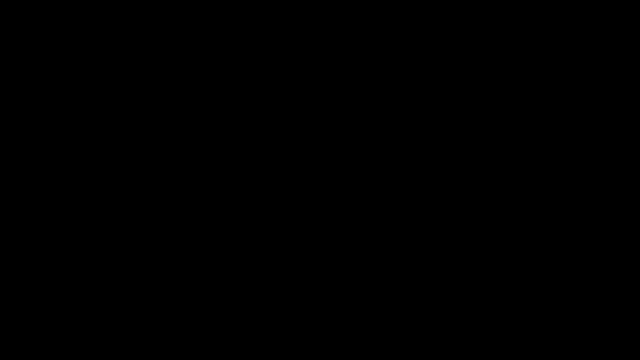 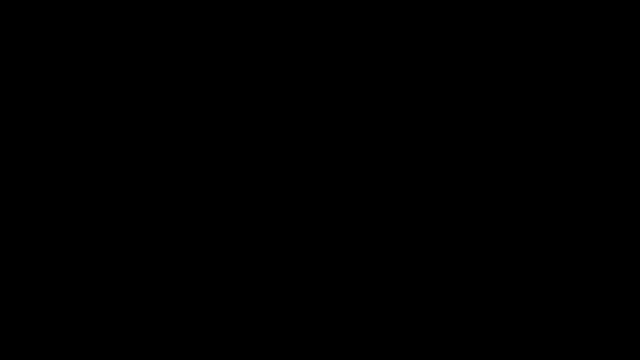 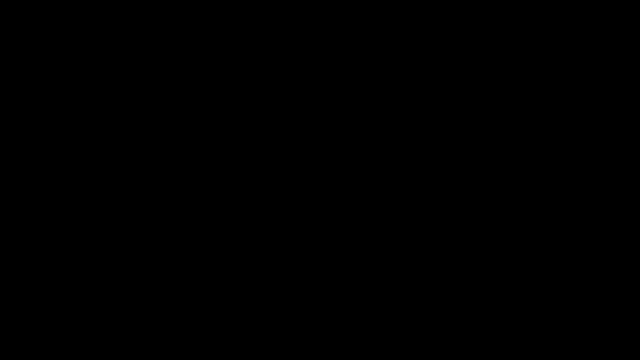 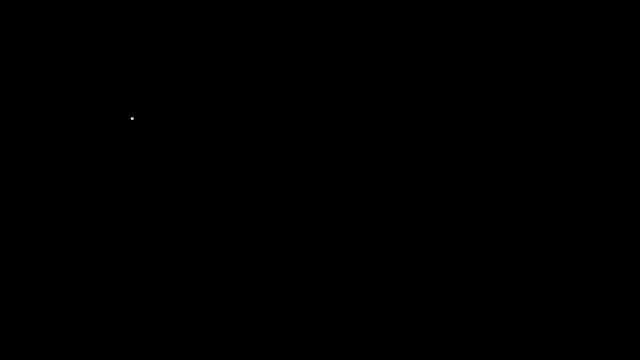 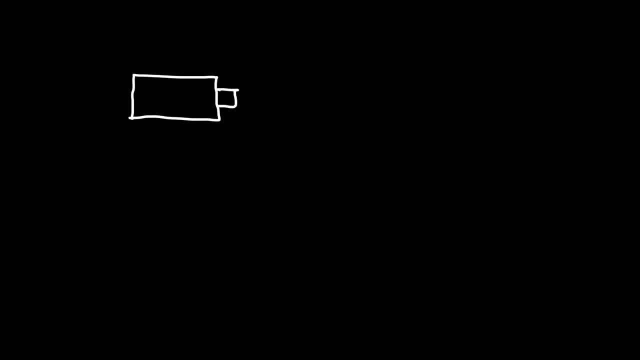 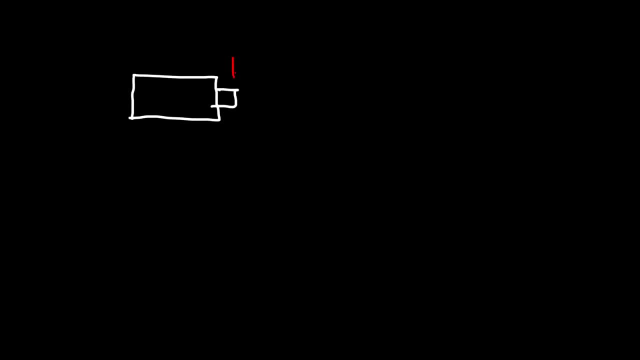 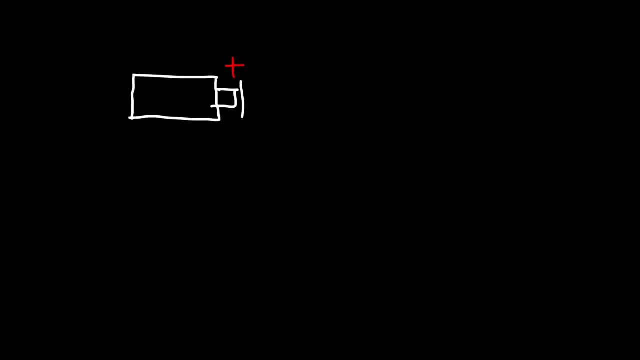 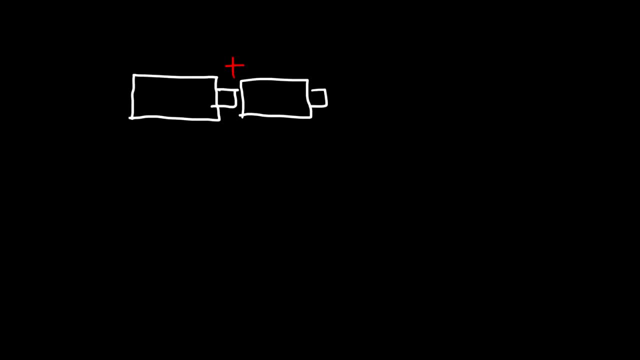 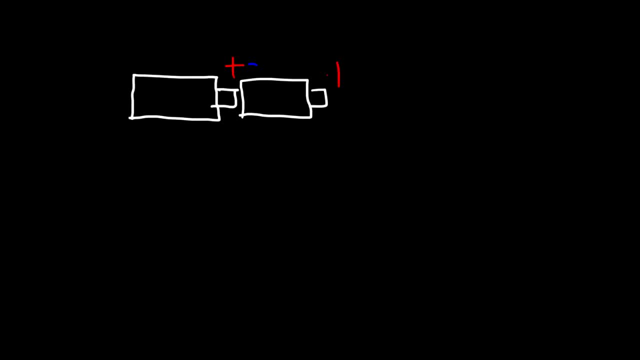 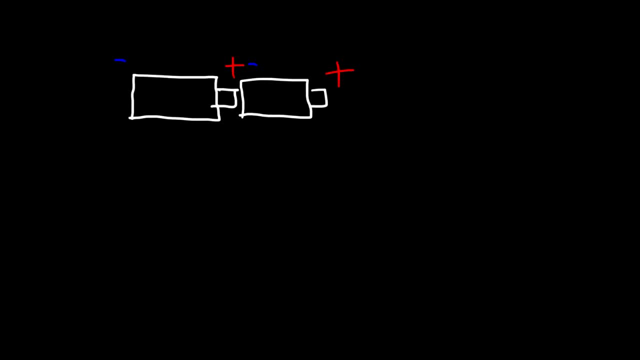 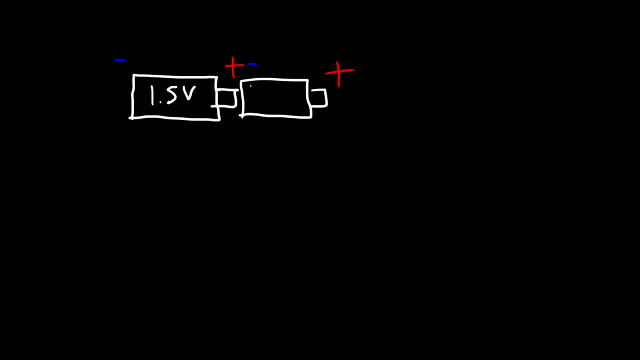 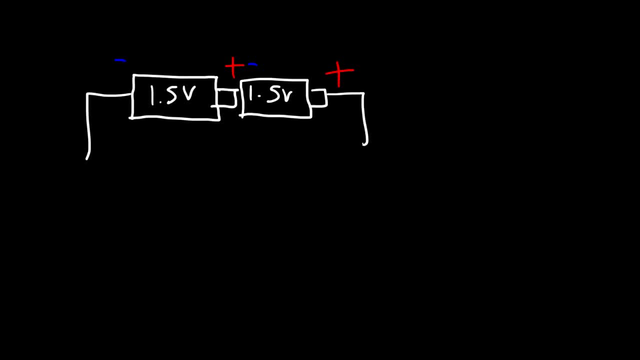 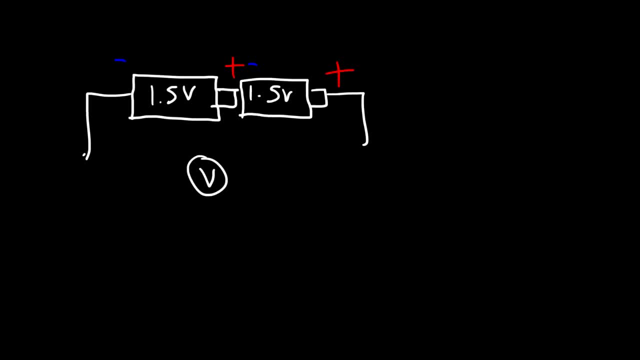 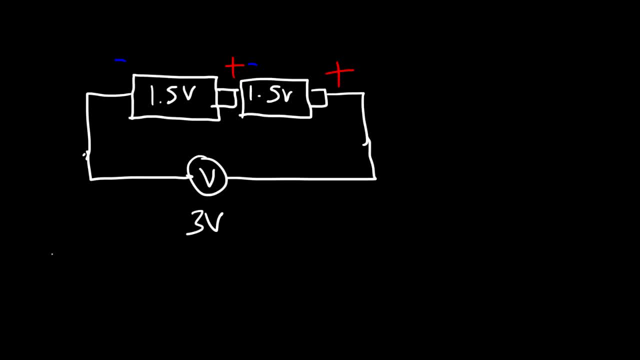 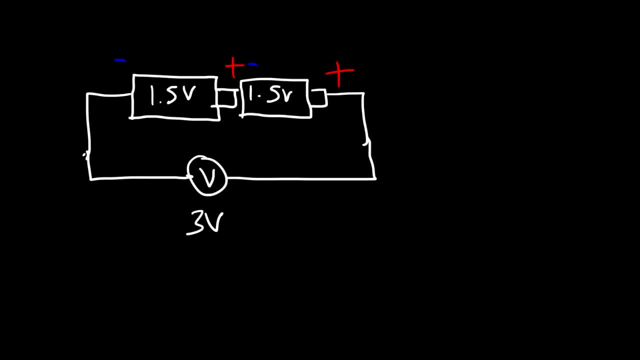 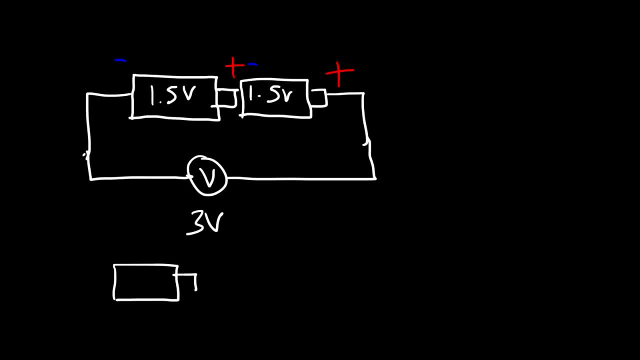 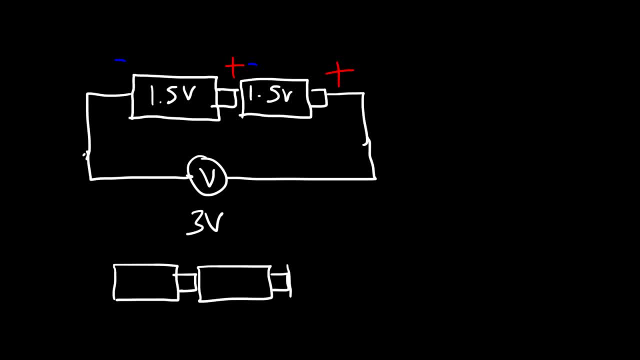 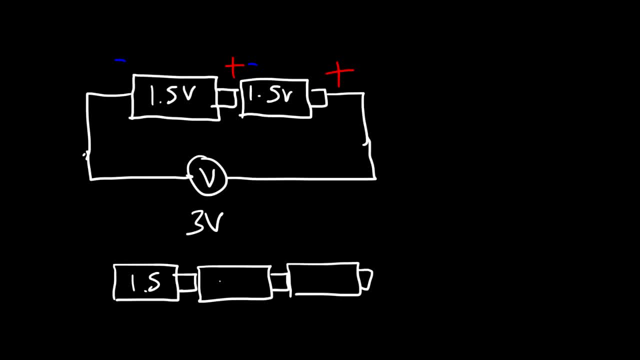 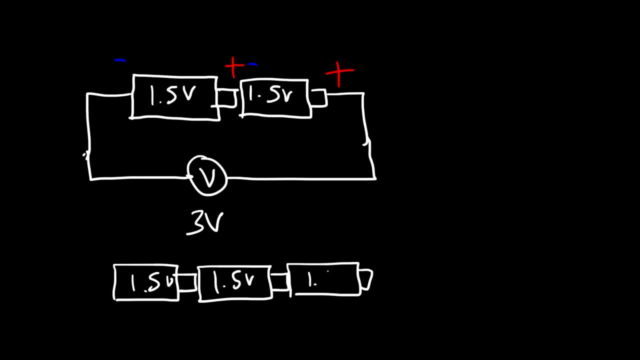 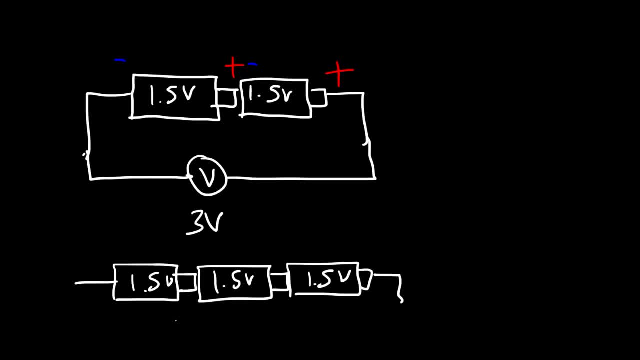 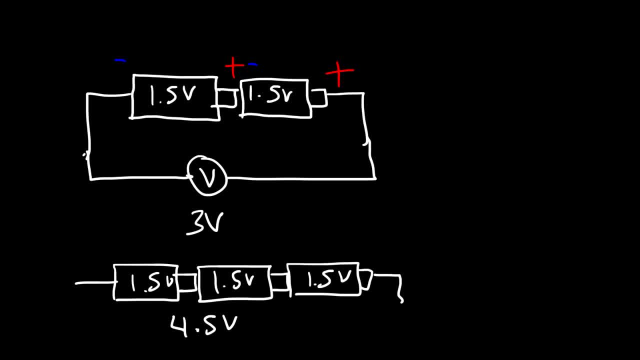 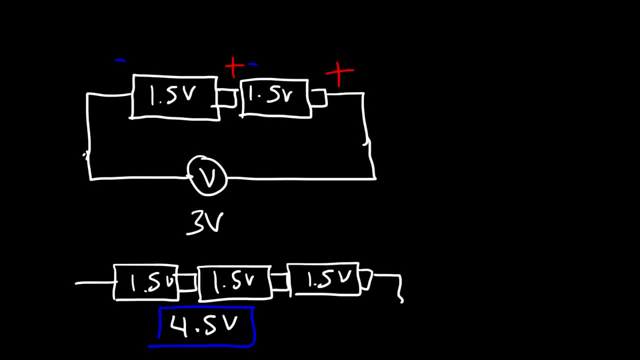 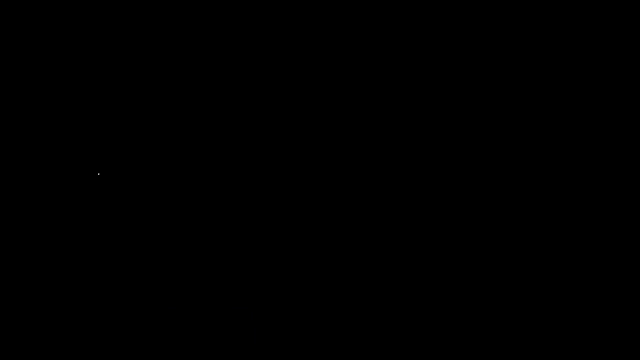 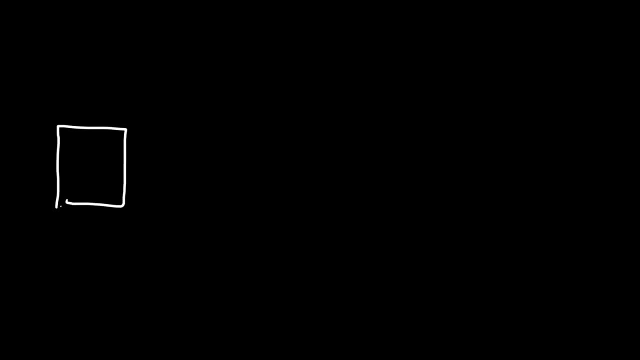 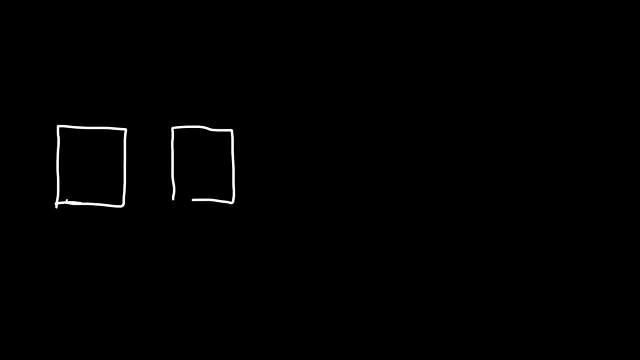 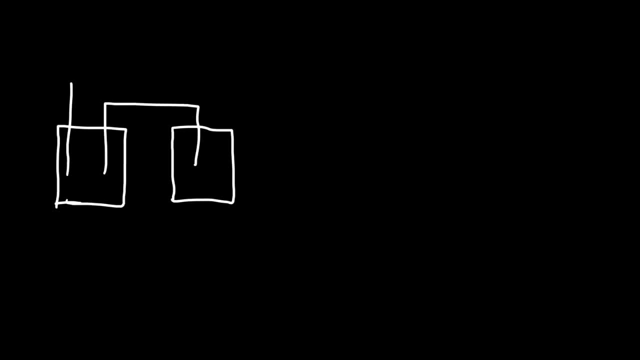 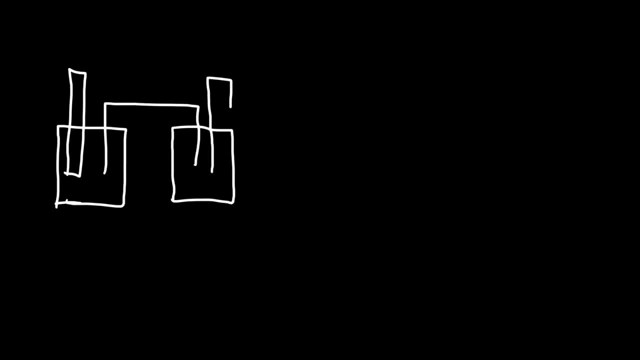 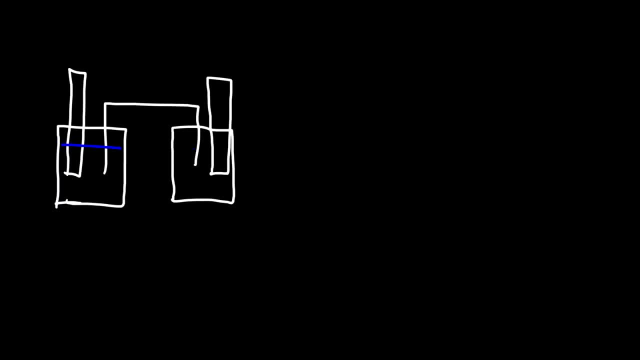 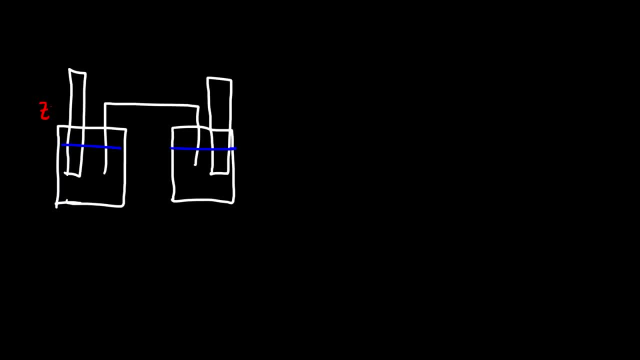 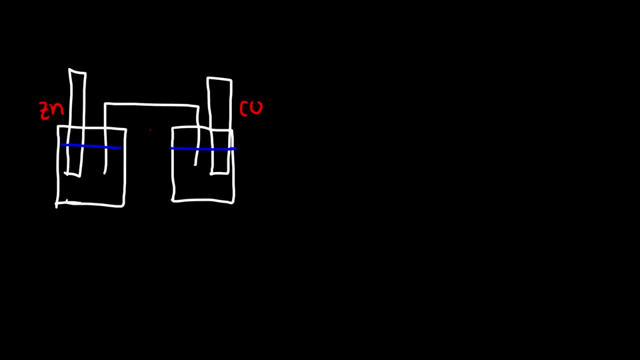 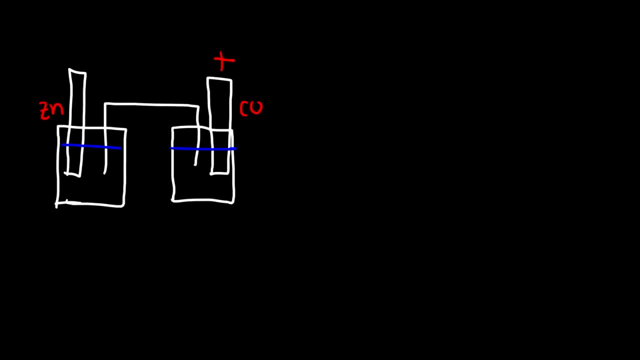 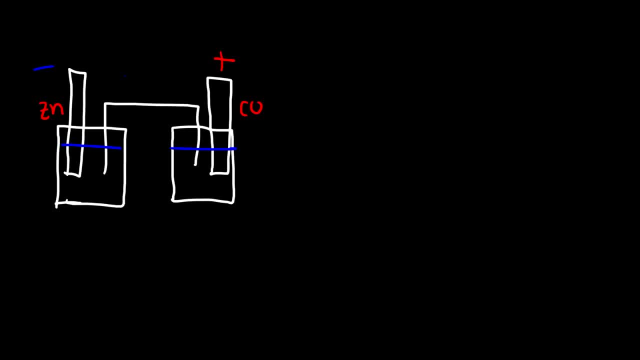 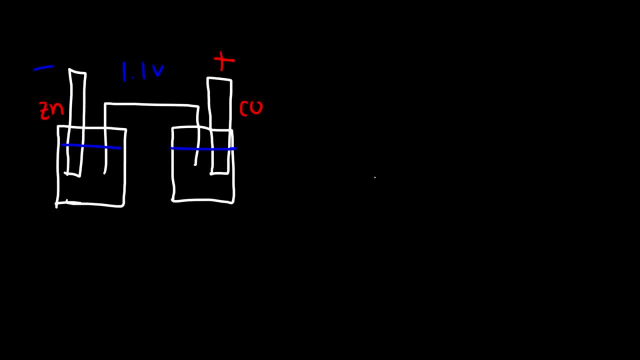 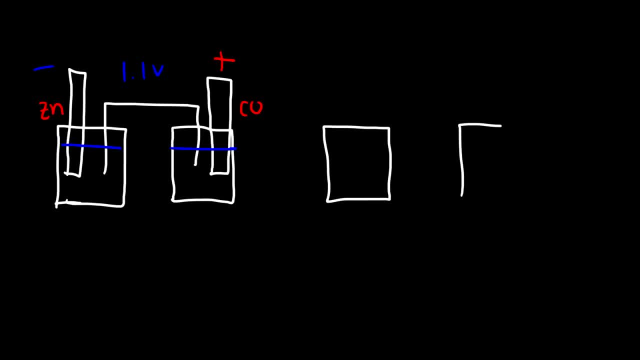 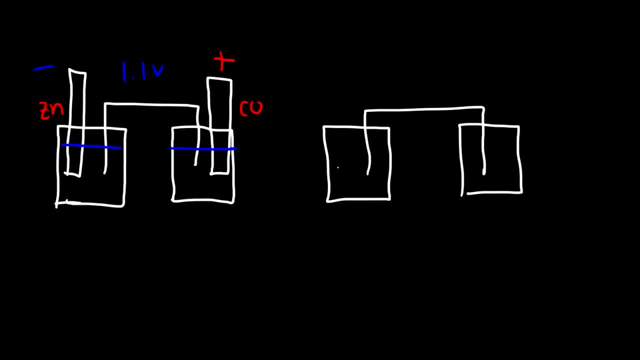 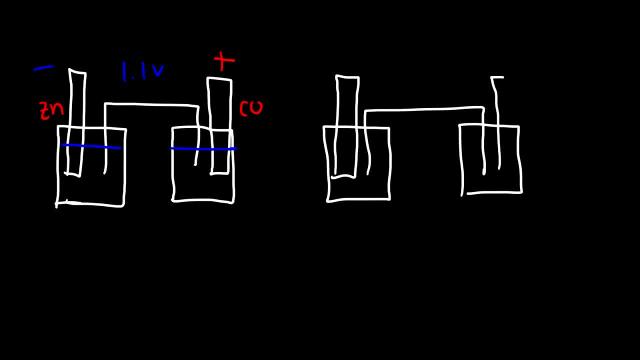 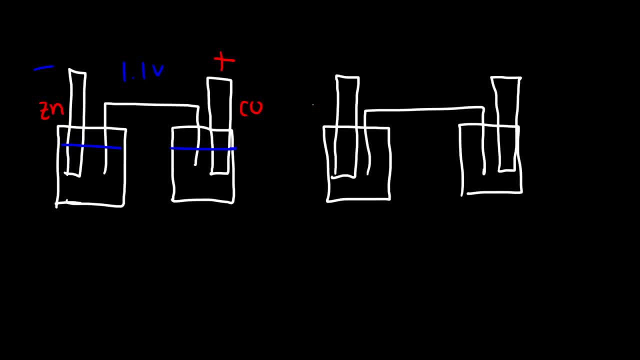 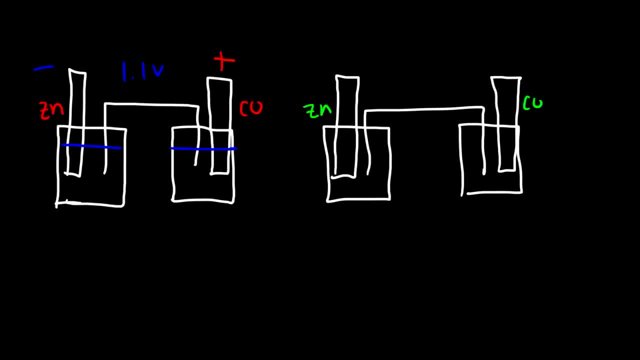 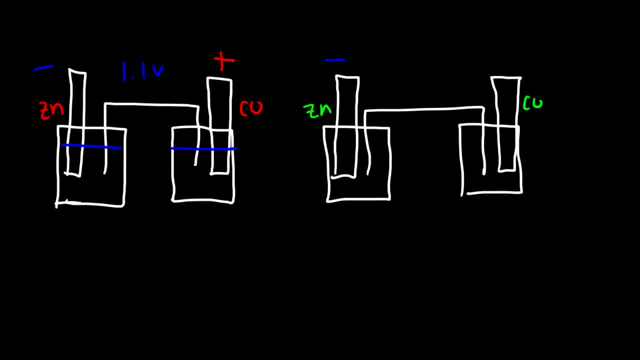 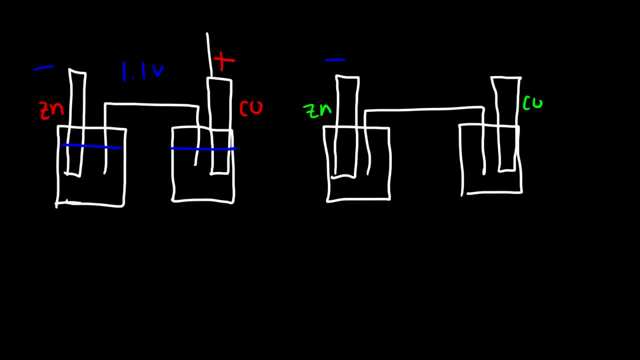 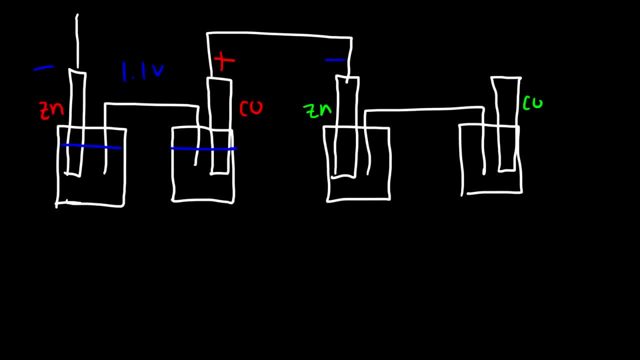 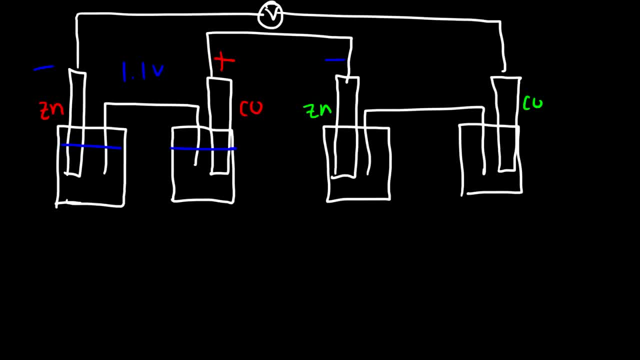 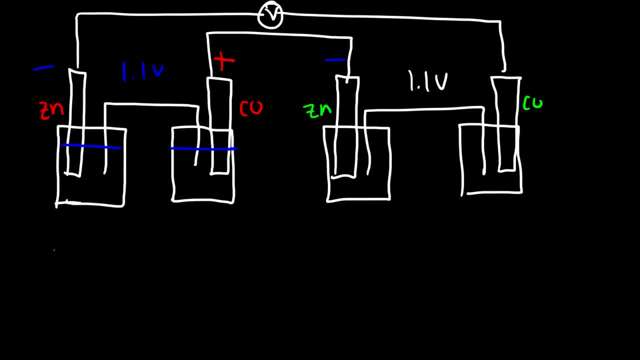 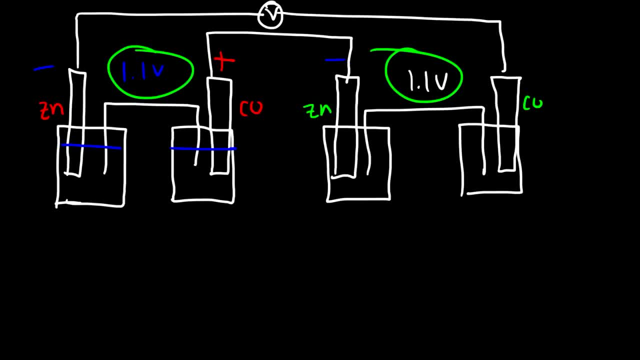 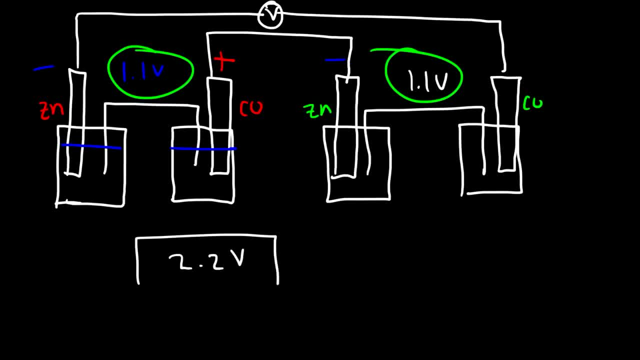 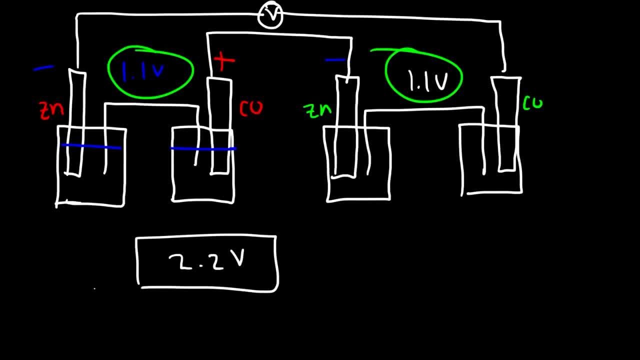 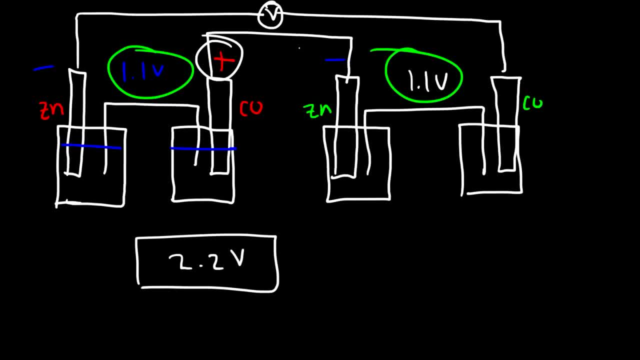 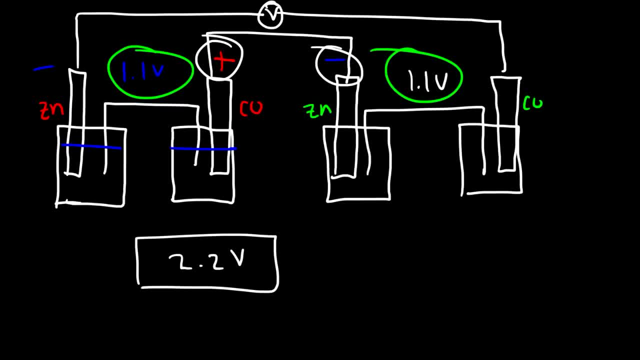 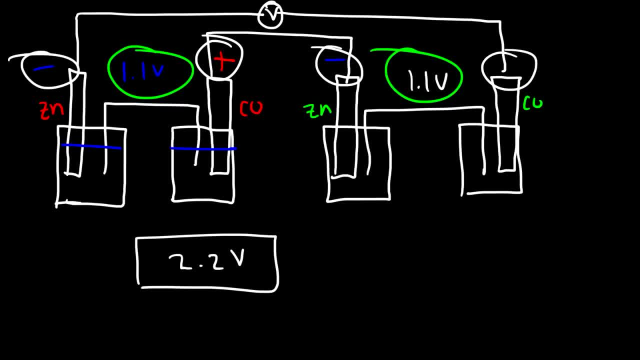 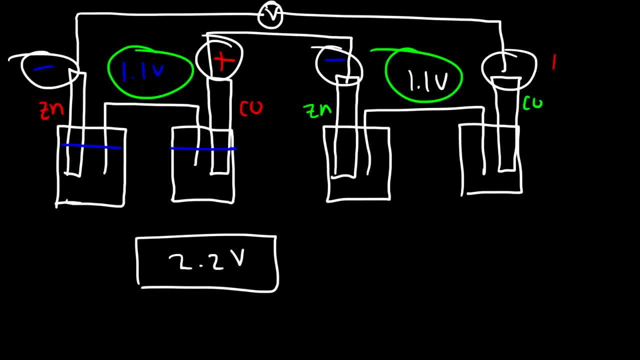 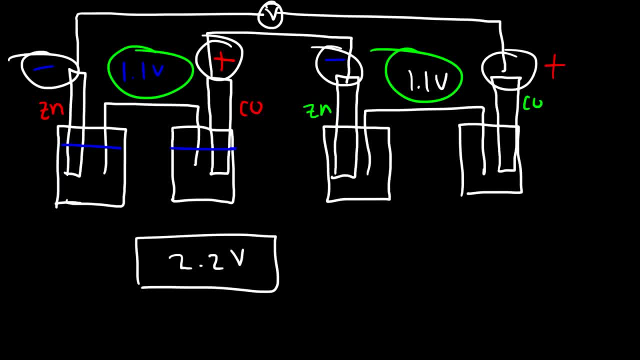 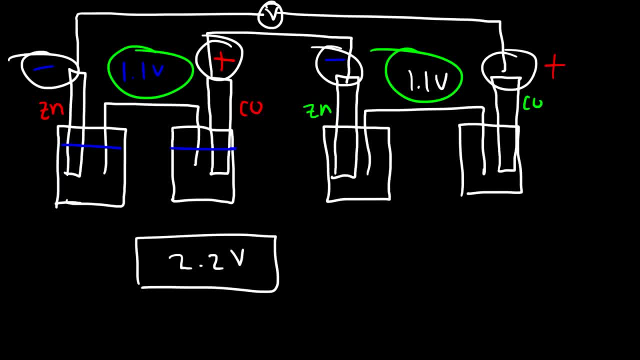 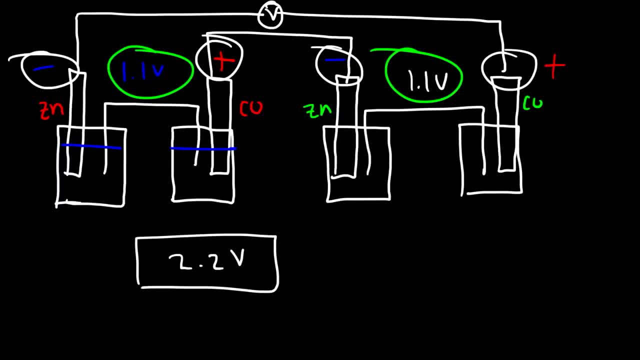 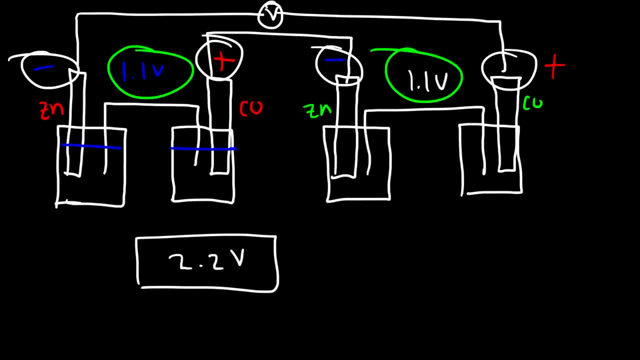 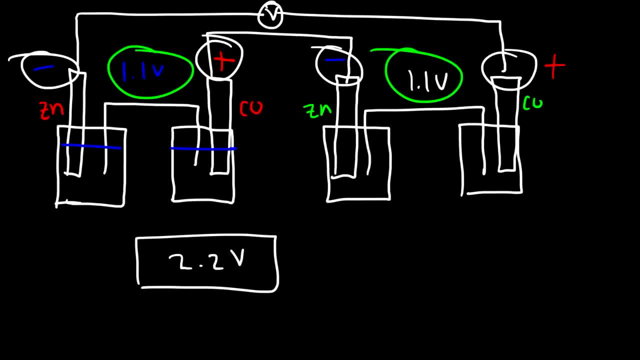 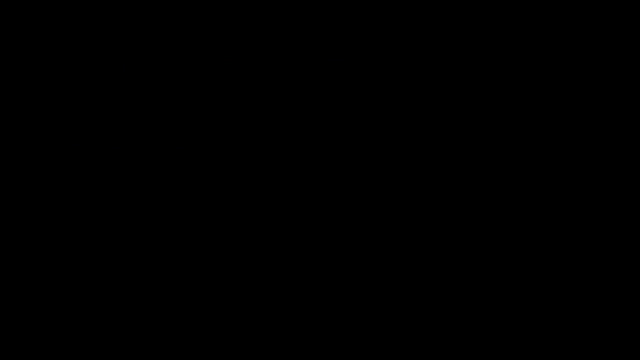 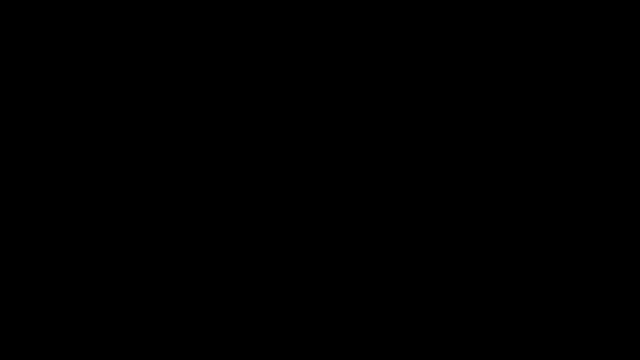 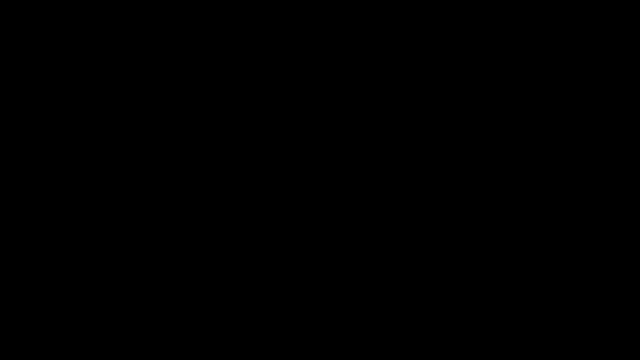 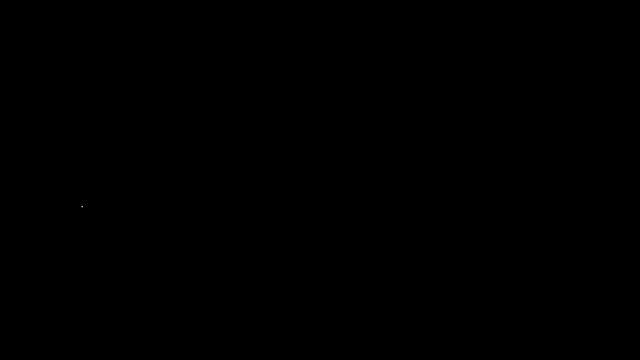 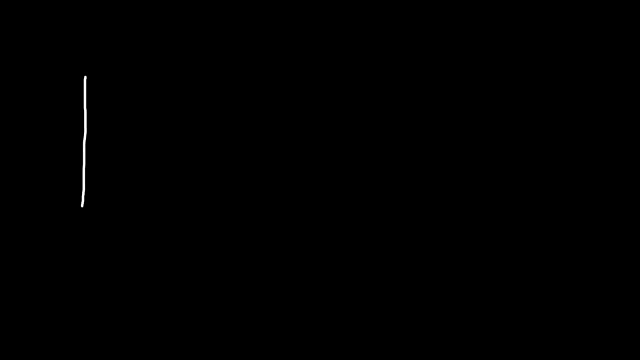 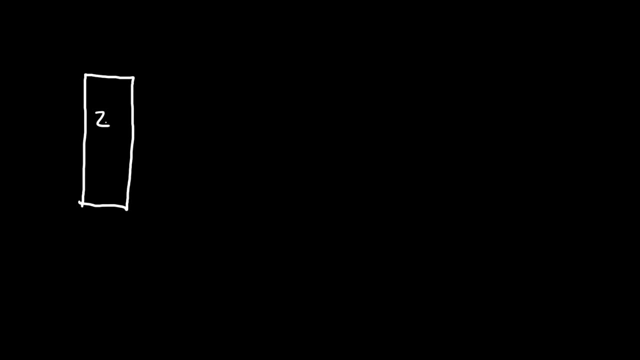 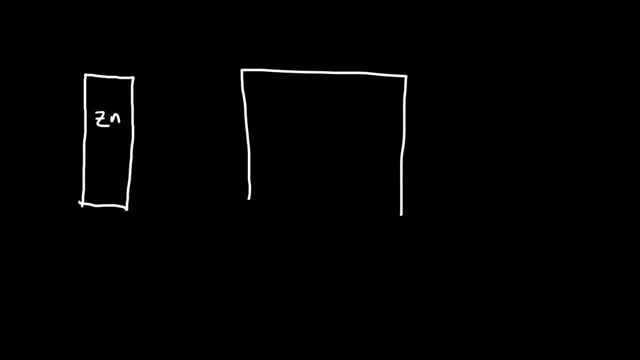 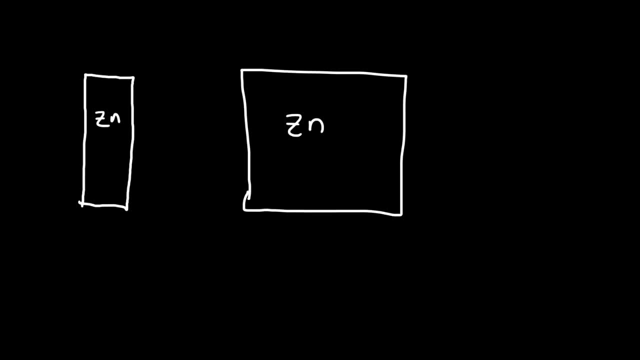 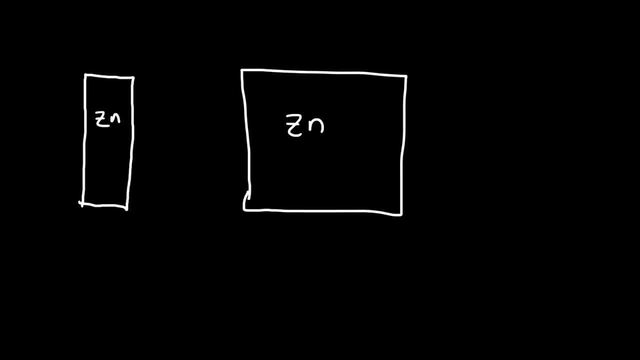 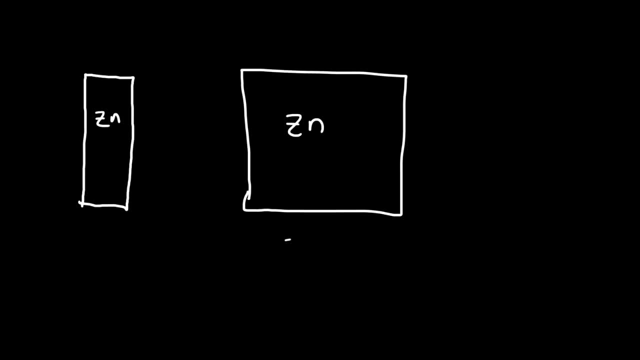 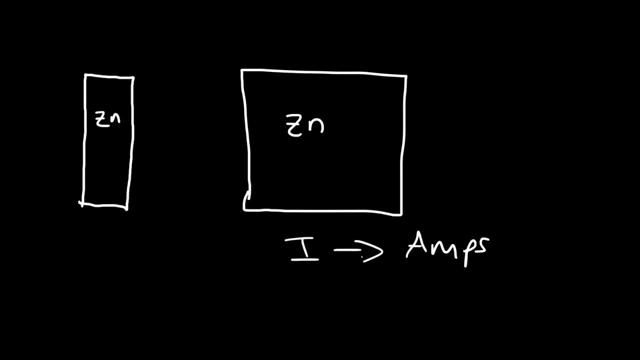 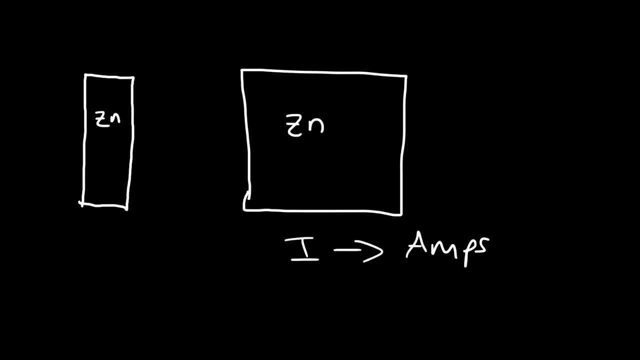 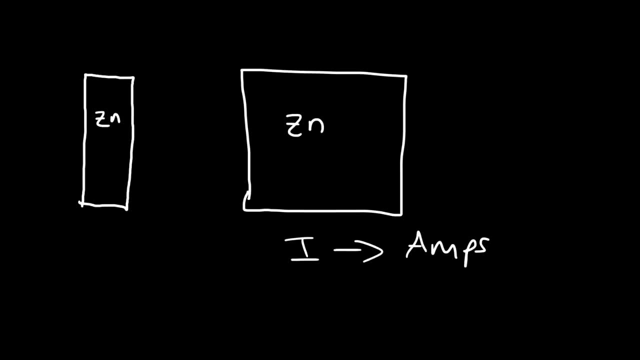 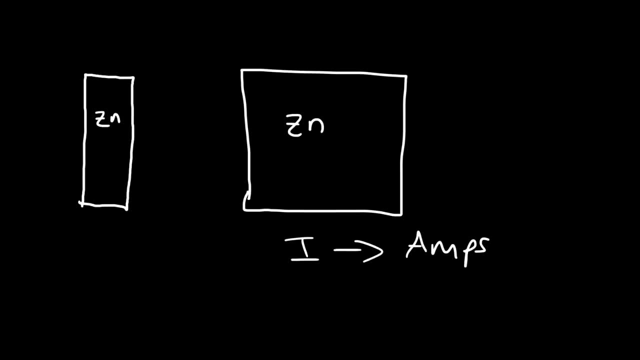 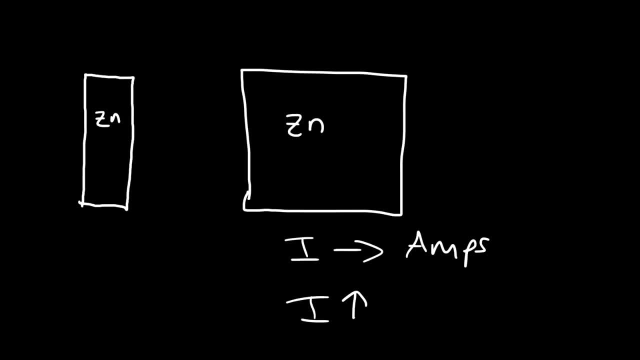 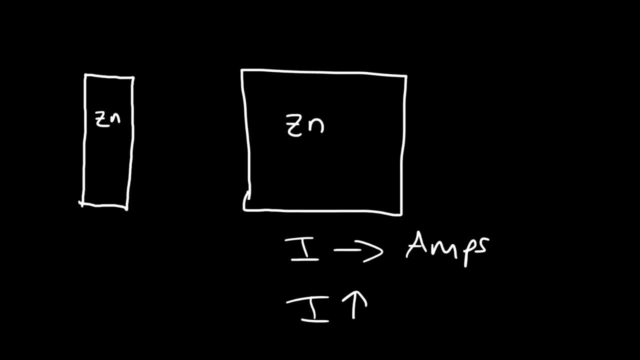 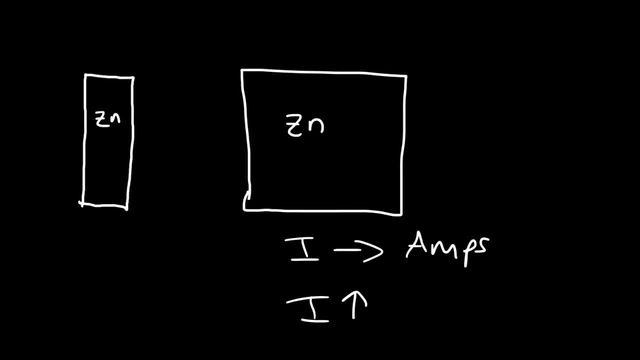 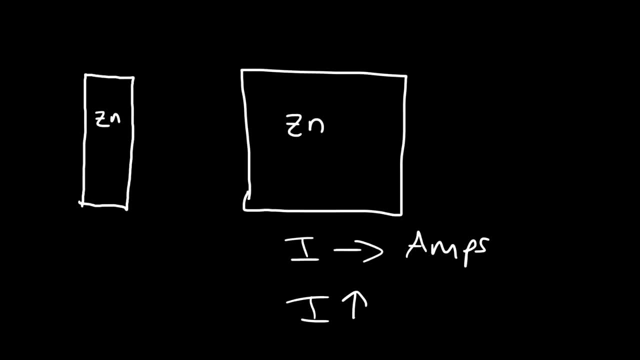 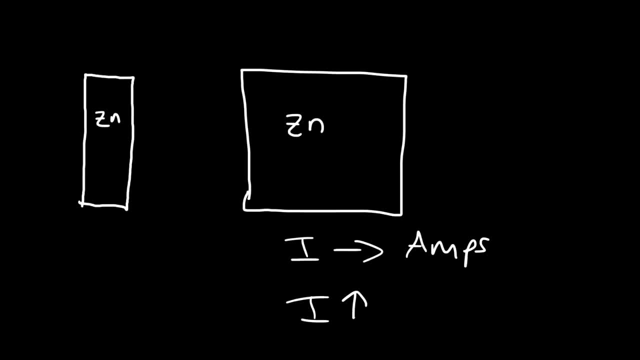 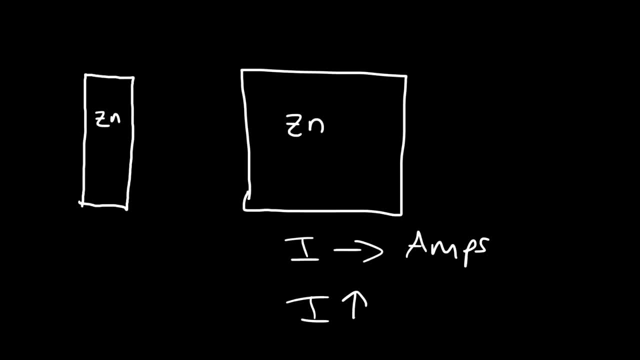 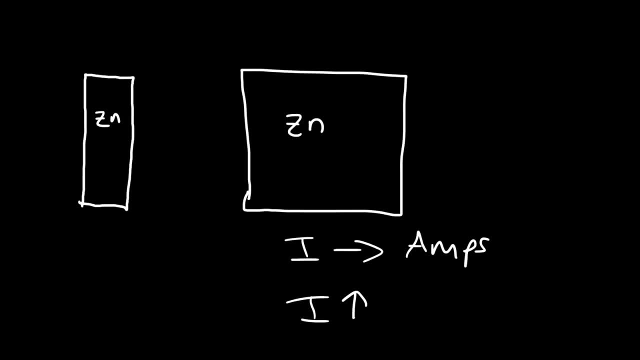 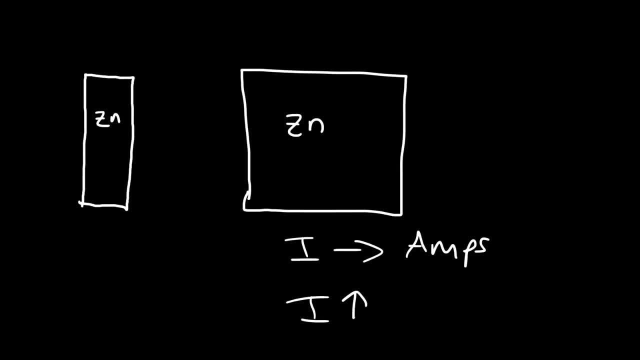 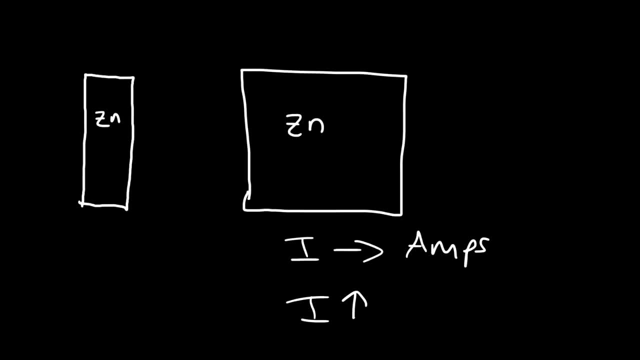 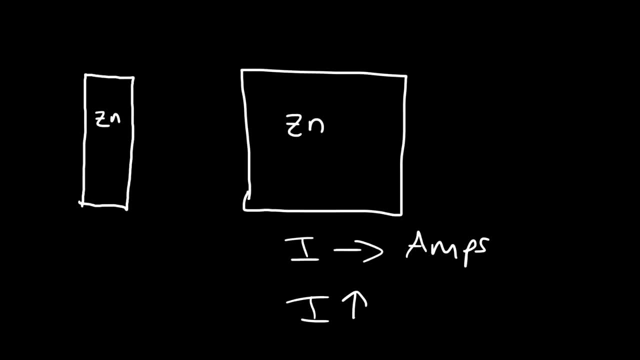 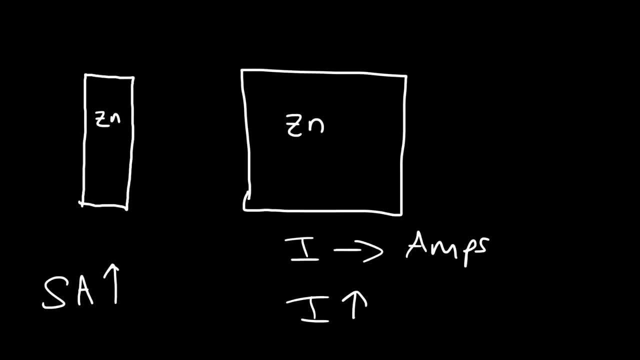 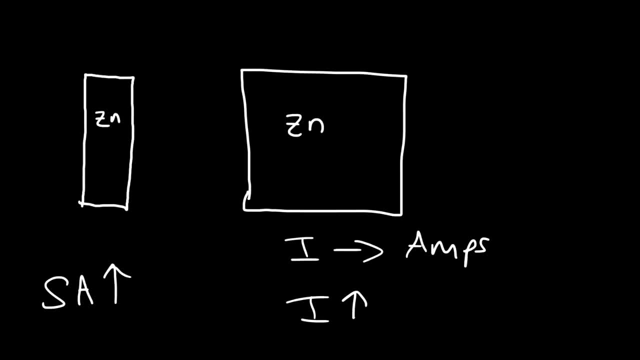 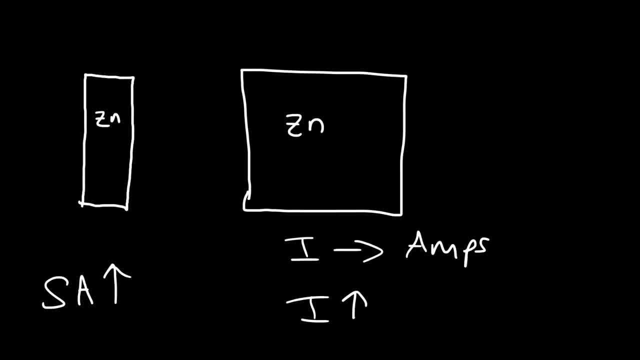 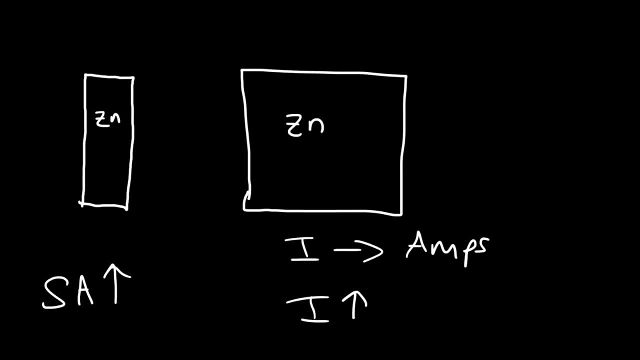 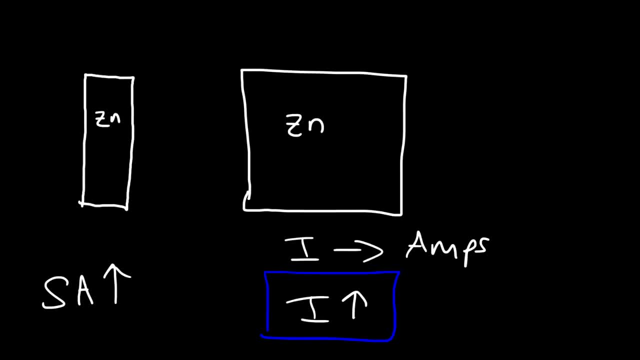 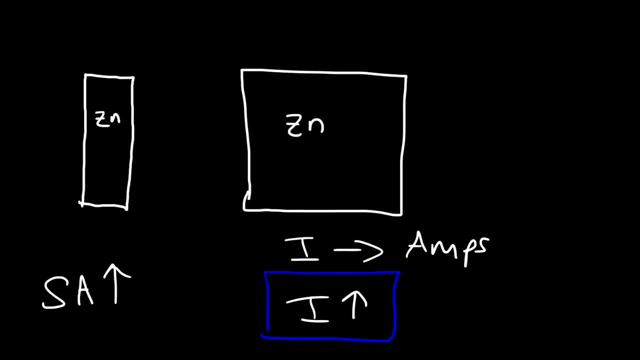 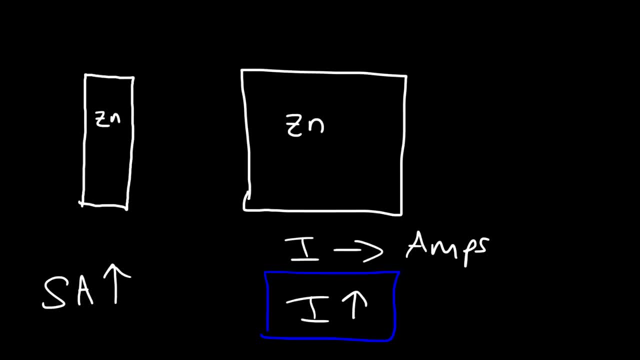 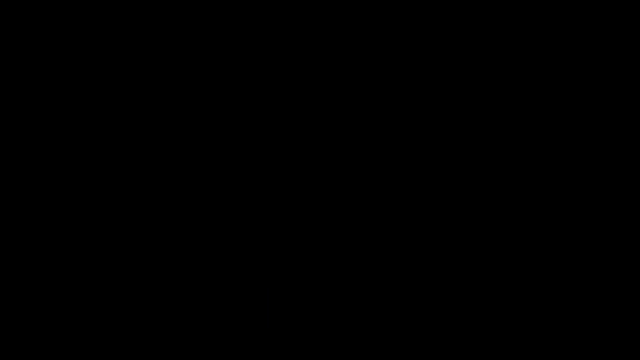 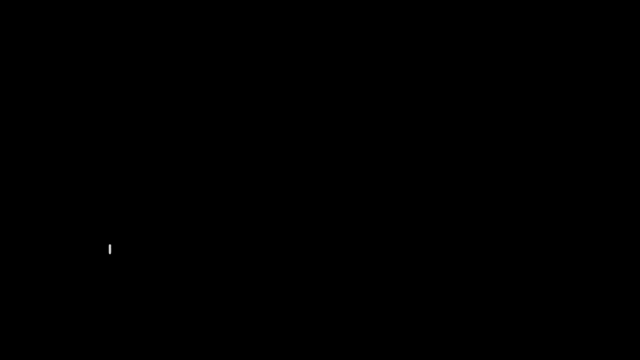 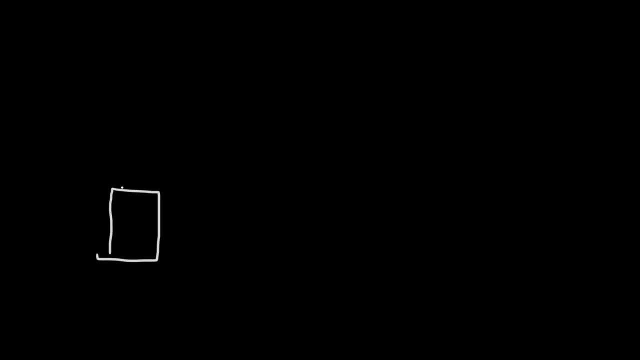 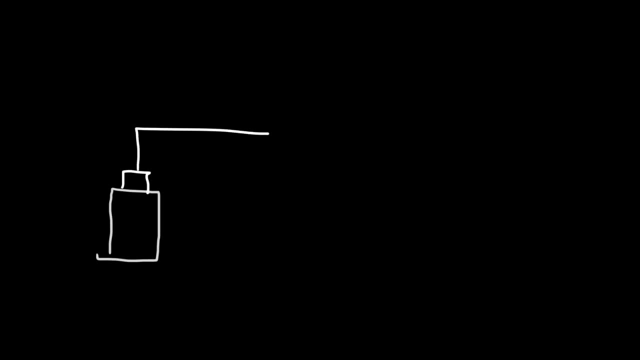 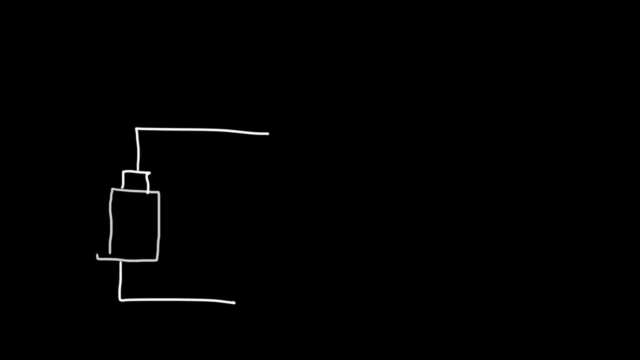 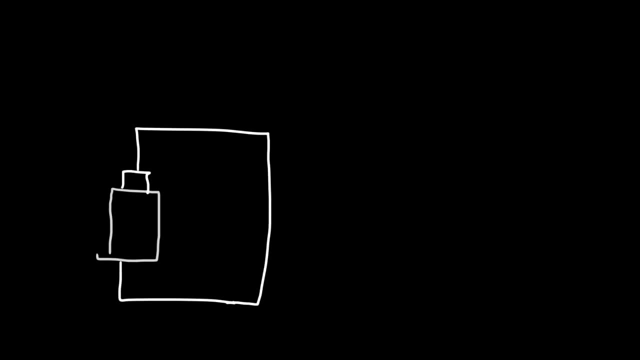 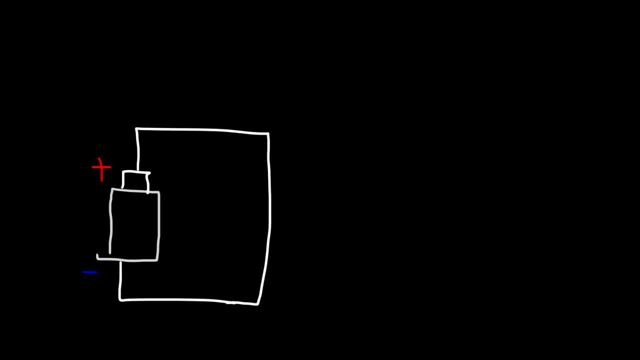 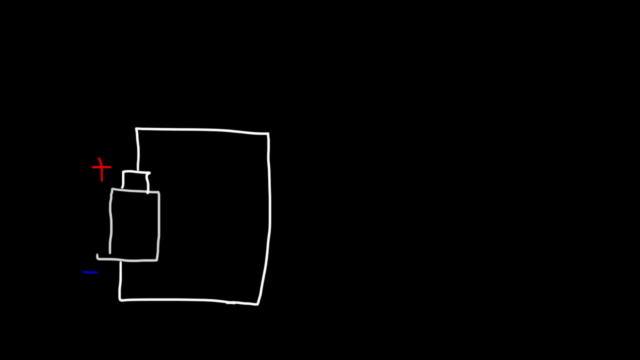 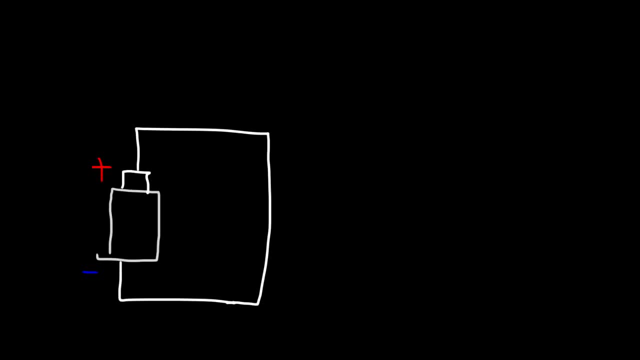 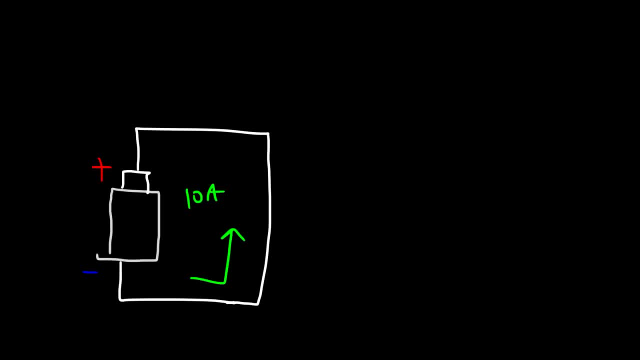 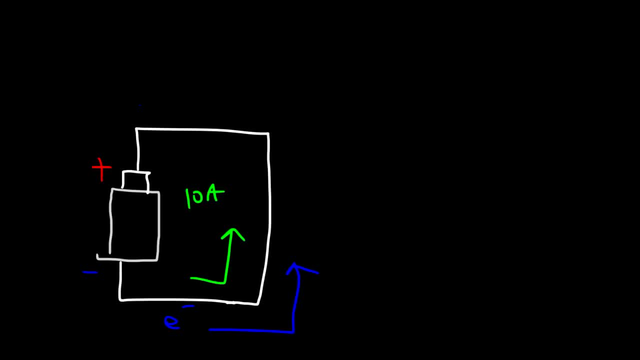 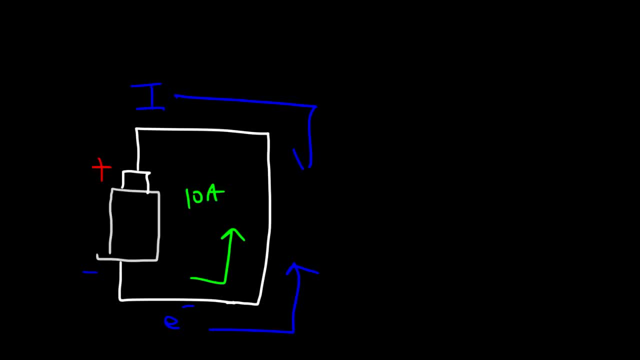 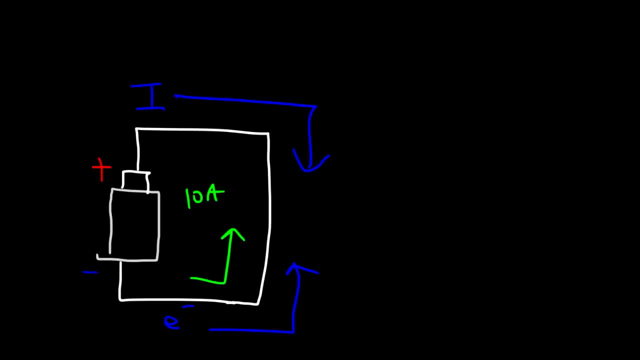 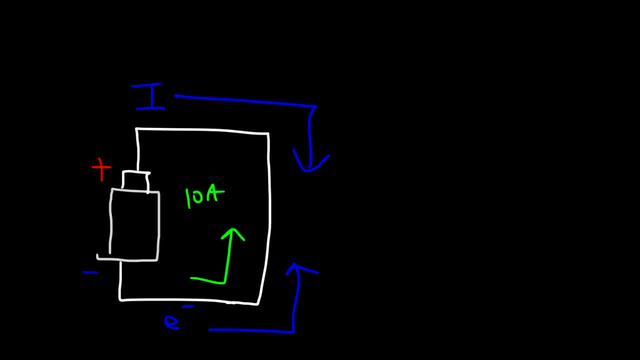 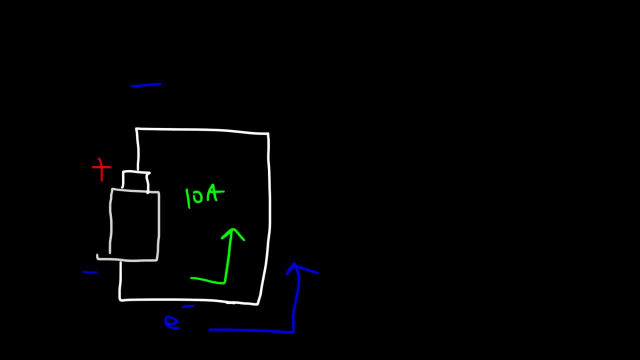 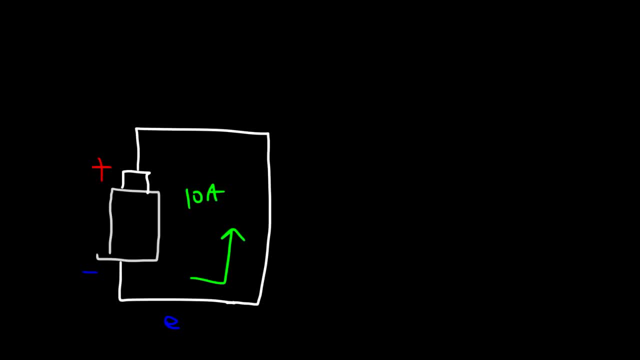 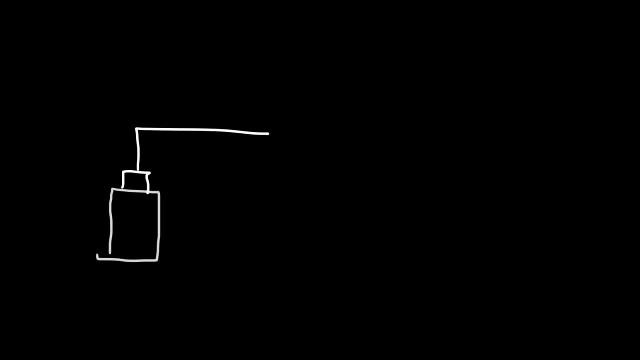 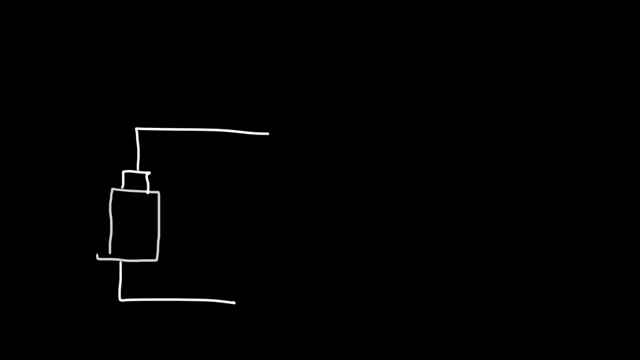 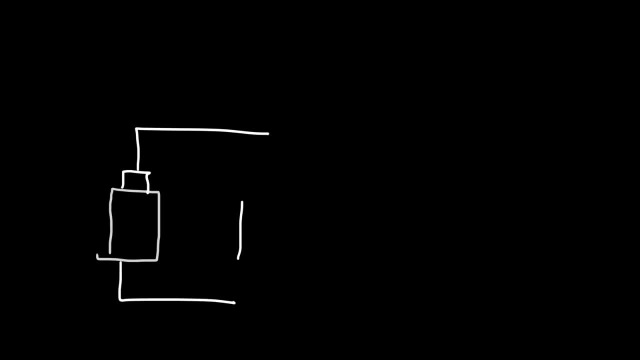 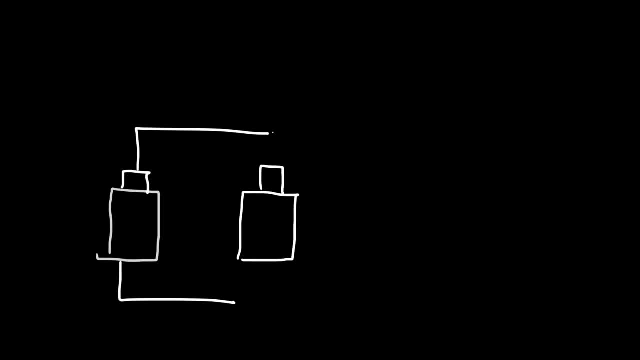 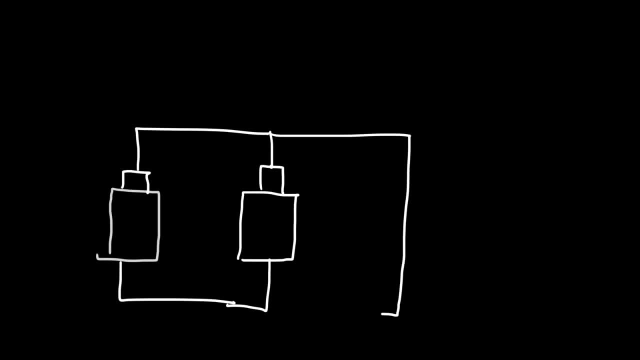 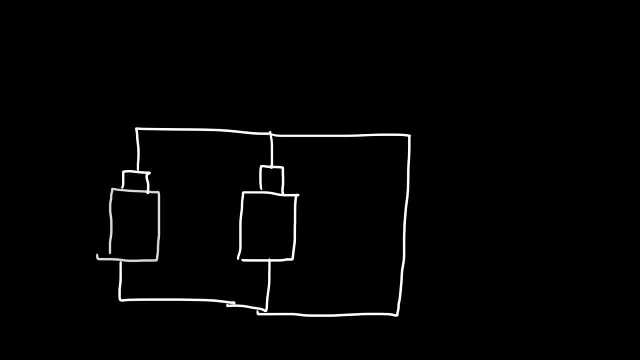